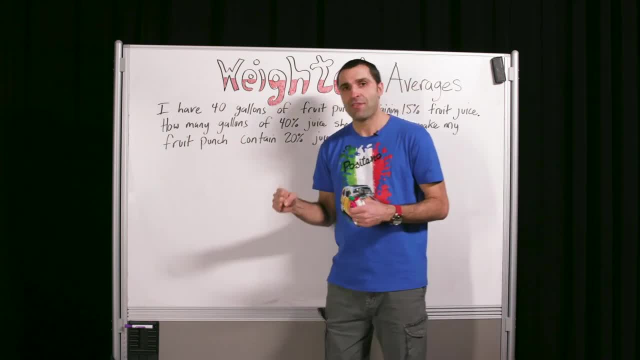 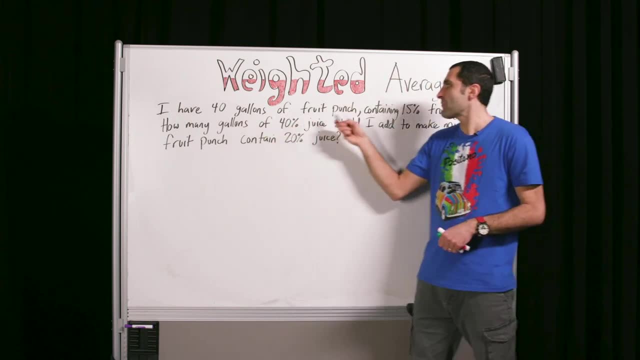 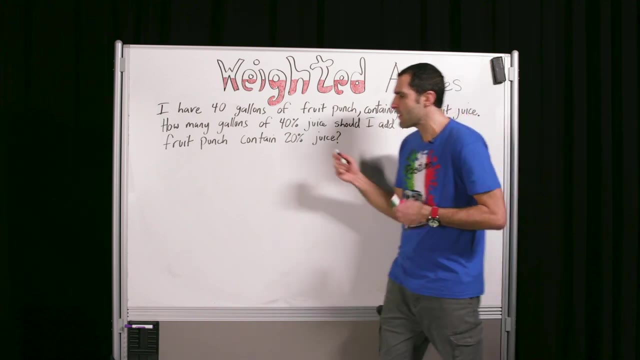 surefire strategies to solve. All right, let's do this. Yay math, Here we go. So imagine, let's say I'm a juice company and I have 40 gallons of fruit punch containing 15 percent fruit juice. So let's just pause there. So I have this like container, you know, let's just 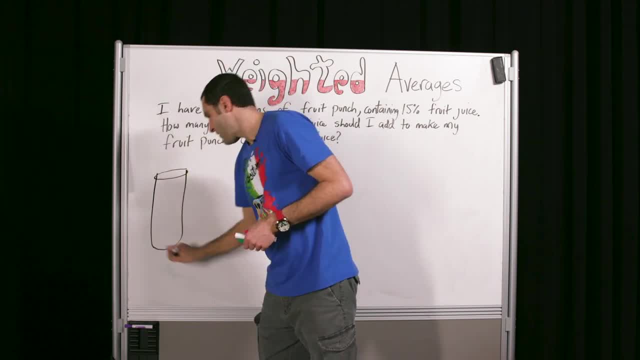 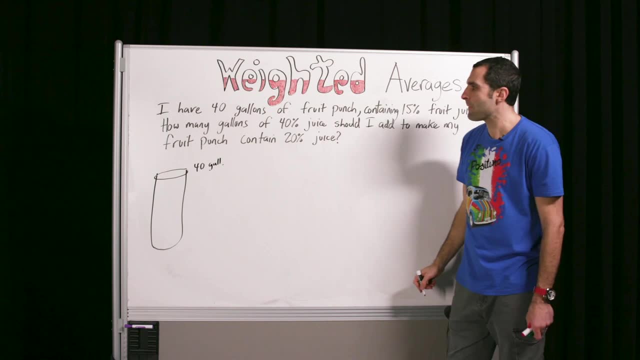 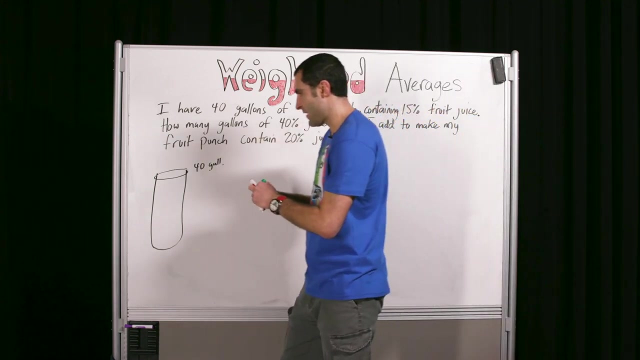 make it like a simple something. simple like this: All right, so this is 40 gallons, All right, and I have it full fill to the top, All right. and then within this mix you could say is like, let's say the full thing is full, like there all the way, fill to the top, all the way. 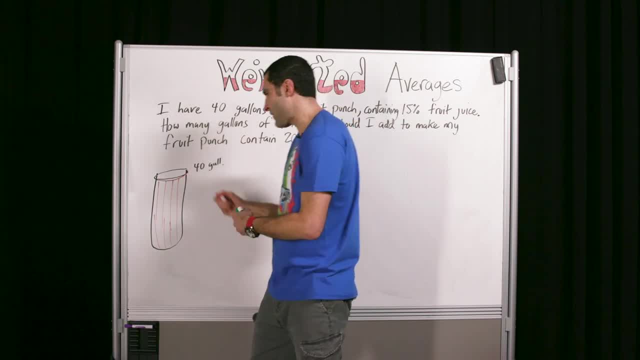 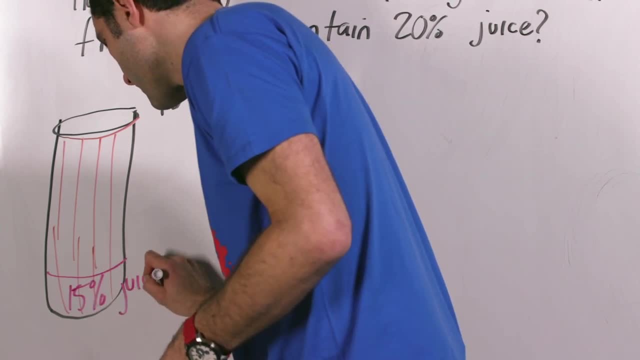 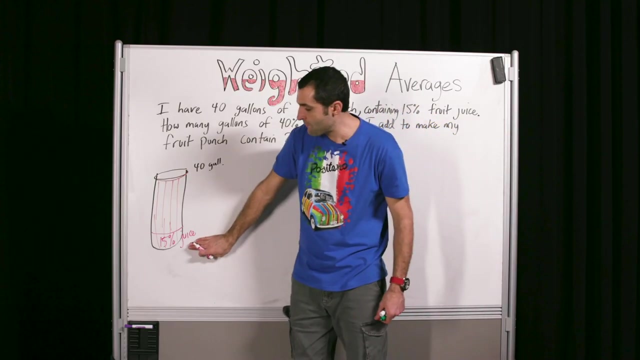 and then within it, though, is 15 percent actual juice. All right, so it's like 15 percent juice. The rest might be water or filler or sugar or color or things like that. okay, But there's actual 15 percent fruit juice in this 40. 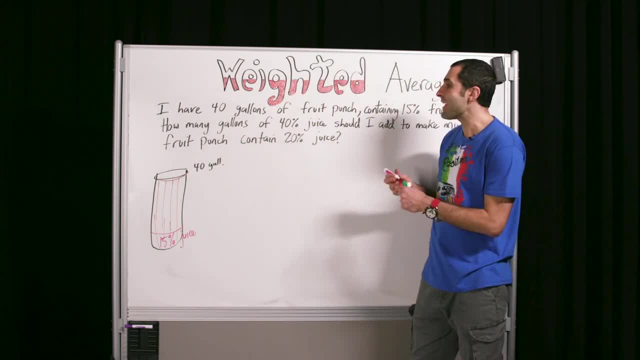 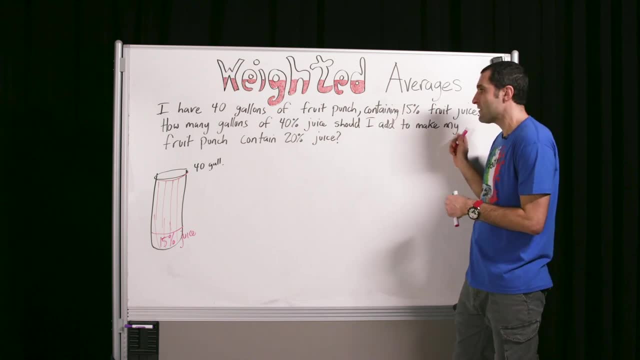 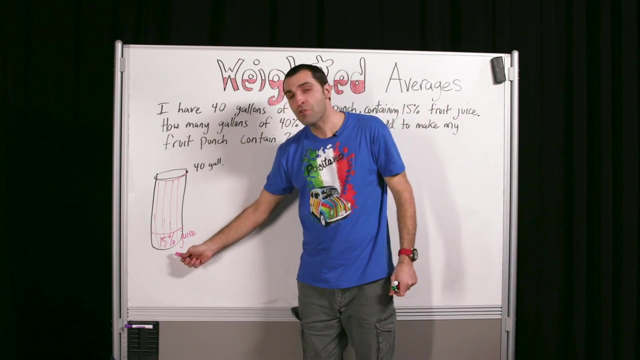 gallon mixture. Okay, how many gallons of 40 percent juice? so, like a higher concentrate of juice should we add to make my fruit punch contain 20 percent juice Interesting? So this juice amount will actually go up. So what we need to do is we need to increase the size of the container. 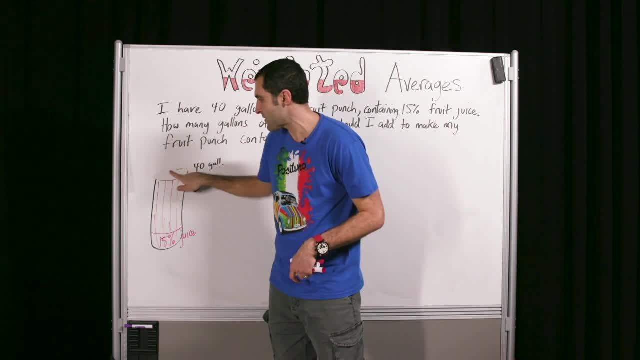 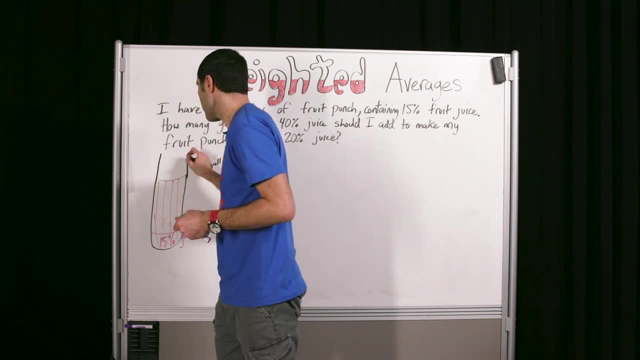 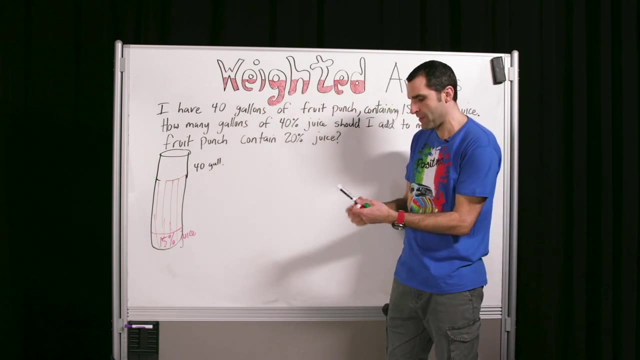 That's for sure. So let's say we still have 40 gallons, because if it's completely full to the top, then we can't really add anything. So notice how I'm just adjusting as I go. you know, there's no problem in that. It's a discovery along the way, It's a journey right? Celebrate that with me. Celebrate. 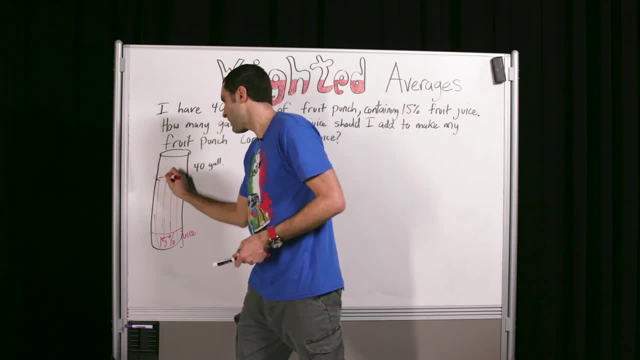 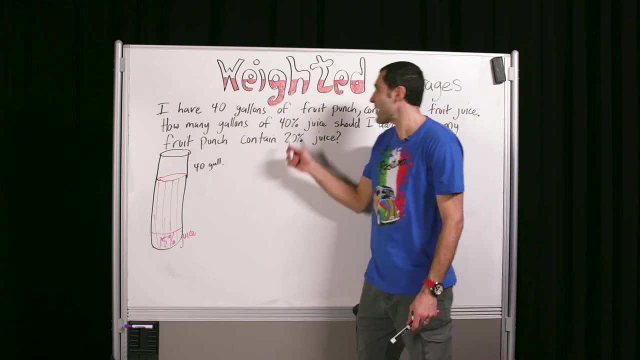 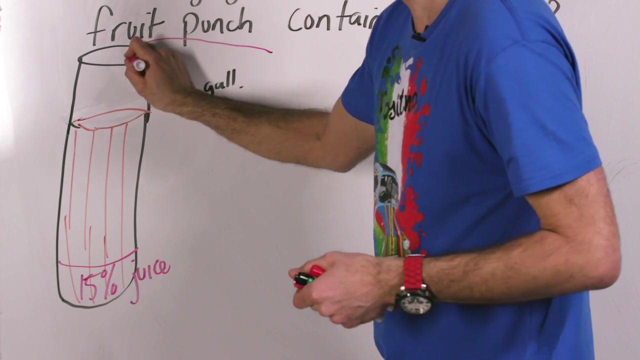 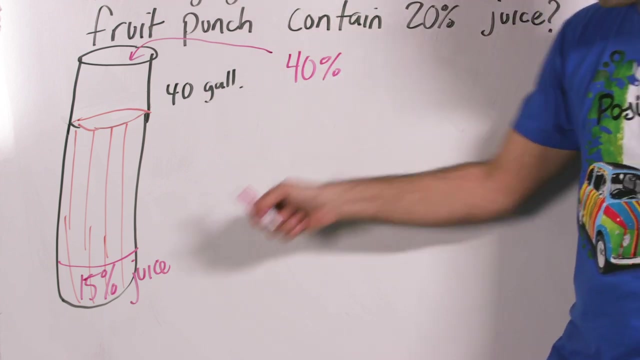 the journey of discovery and it's going to work out there. So we still have 40 gallons in this larger container and I want to start to add 40 percent juice, So like this new juice coming in, All right, so dumping it in in there and that's like 40 percent. So you see, it's more concentrated. 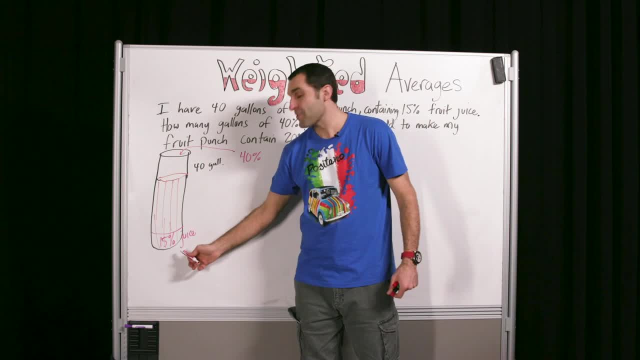 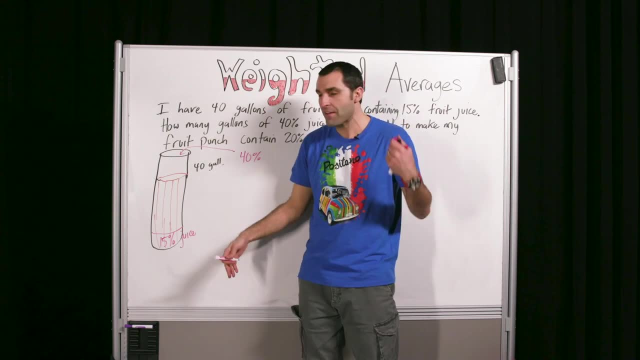 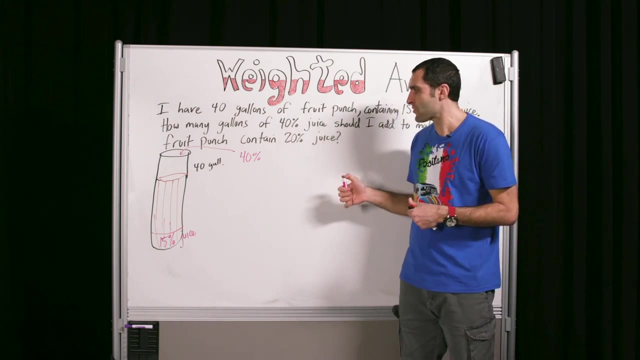 than the 15 percent, and so over time the percentage of juice will go up. It'll go up to like 16 percent overall juice in the container, 17 percent overall juice in the container, 18,, 19 and our goal is 20 percent juice. All right, so I hope that helped you understand the problem that we're trying to. 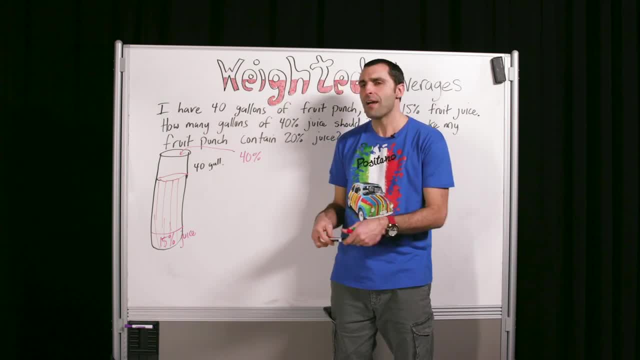 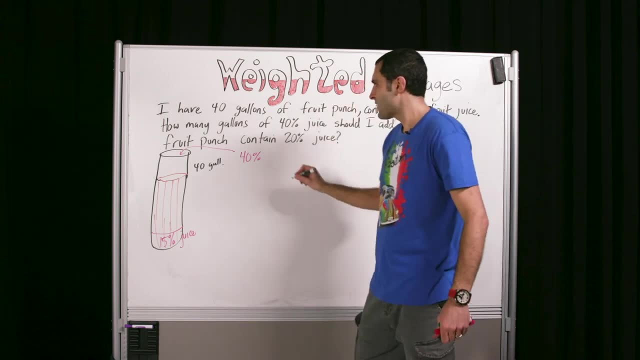 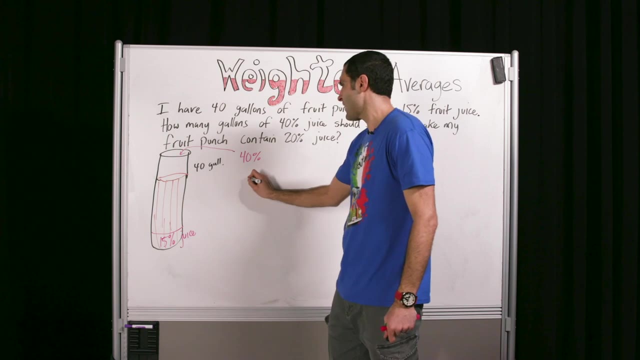 create a, a, a thicker juice content. So how do we do that? Okay, what we need to do is we need to create some sort of ratio. Okay, so you could say, like the ratio essentially is the amount of juice relative to the total punch. Okay, so let's try that. Let's say, like, move this over here, So 40 percent's. 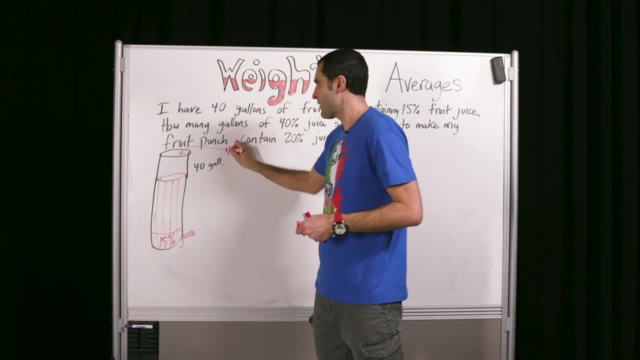 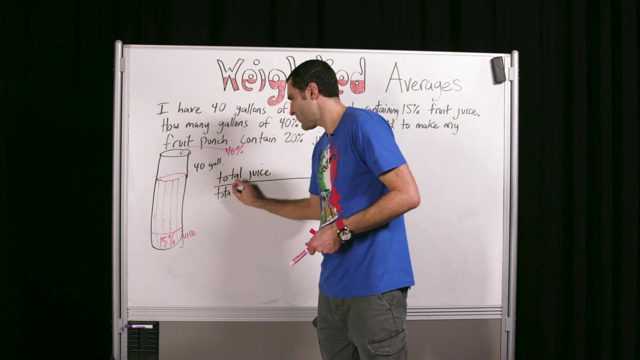 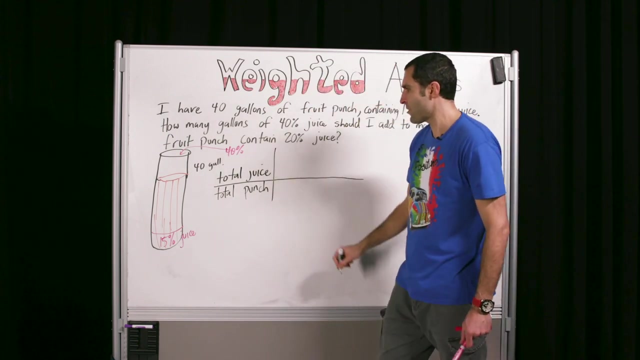 going in. So use that space wisely. for us, 40 percent. So let's say we have total total, total, total total total juice over over total over total over total punch, punch, punch. So we have this little ratio going. So we have this little ratio going. 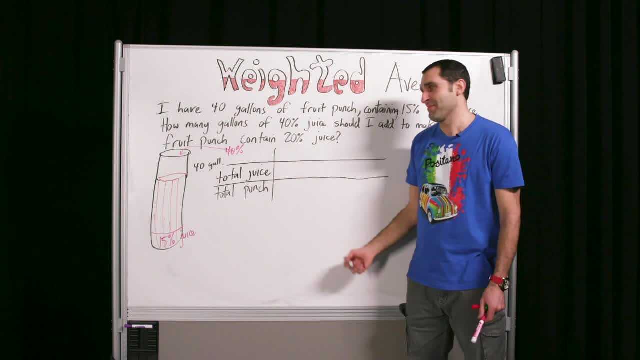 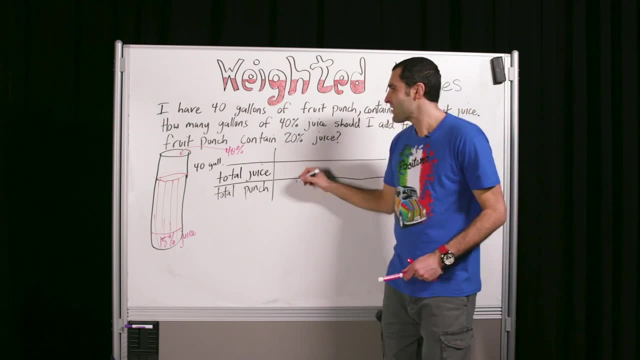 When I've worked with students on this and they say Not the juice problem, they mean not the juice problem, but really like let's, let's really try it together, let's try it okay. so we have first the. what kind of juice? we have the 15 brand, all right, so let's do the 15. 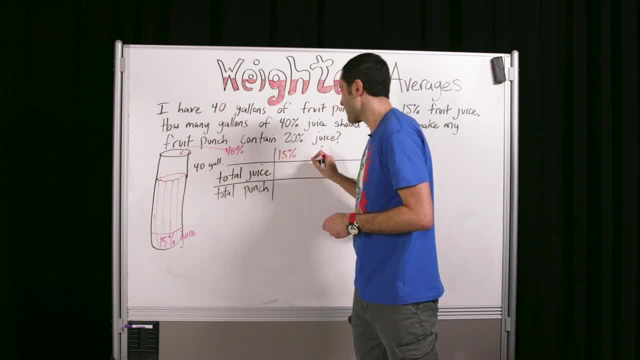 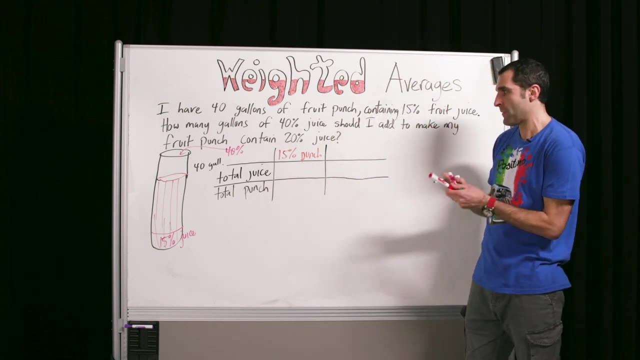 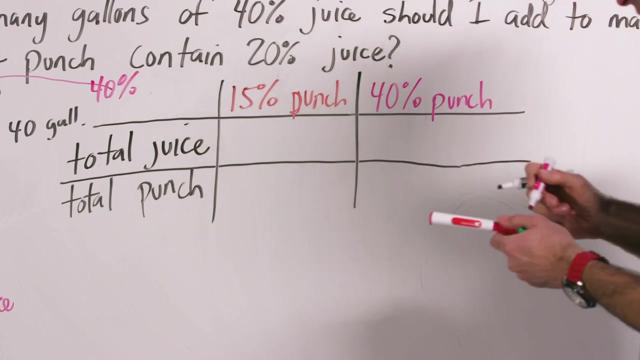 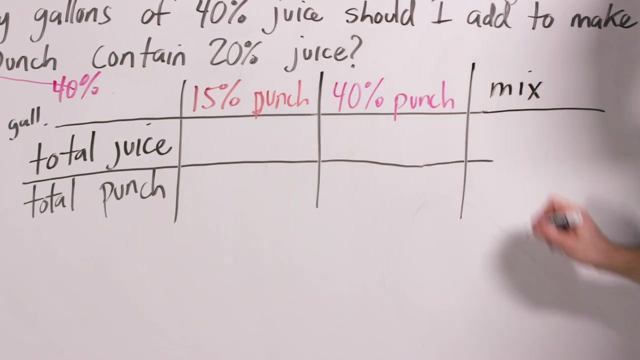 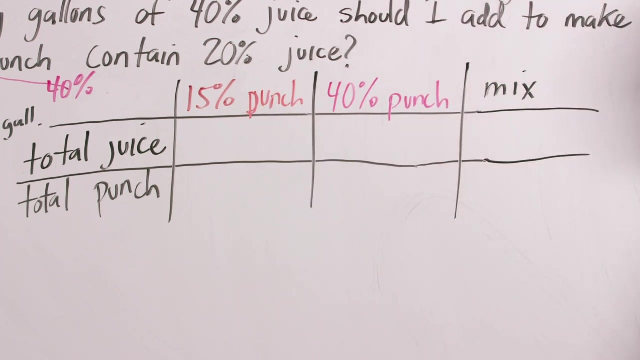 is right. here we have the 15 juice problem. 15 punch. you could say: okay, then we add to it, we add the 40 variety, make that pink 40 punch. we have that kind and we have our mix mix total. okay, so let's see, see it. with regards to the 15 punch, i know how much punch we have 40. 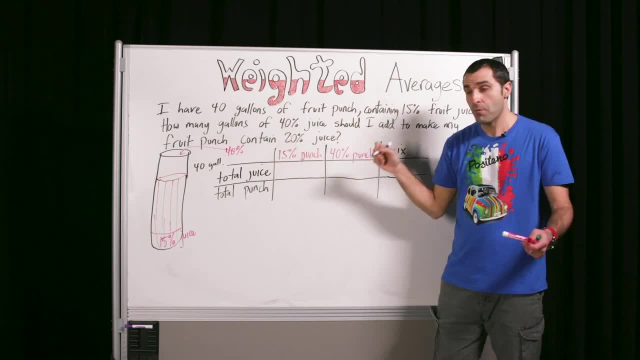 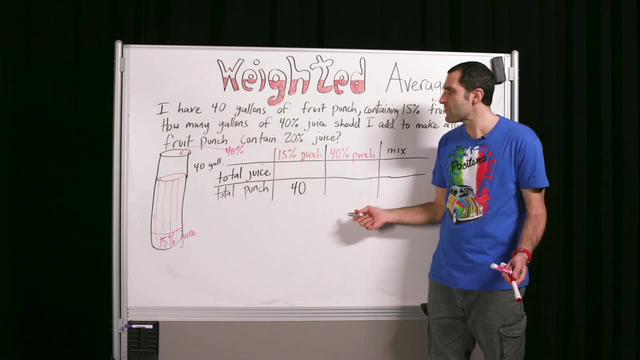 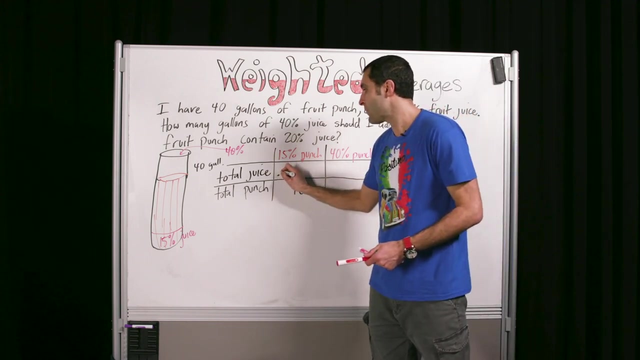 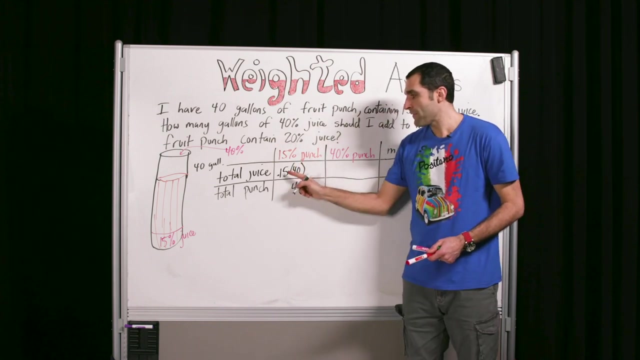 i have 40 gallons of the fruit punch, so we'll put 40 down within this 40. how much juice is that? how much juice? well, i know it's 15 of this, so what i can do is i could say 0.15, which is 15 times 40.. because of the 40, 15 of those 40 gallons is actual juice. 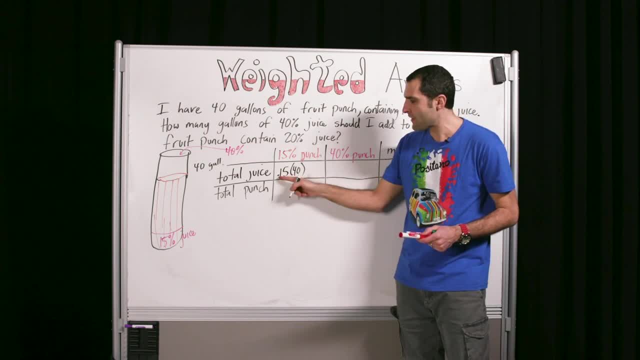 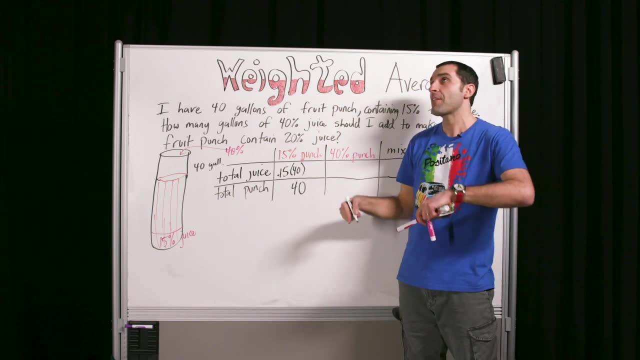 right and if i wanted to to multiply through, I could do a distributive style: 10% of 40 and 5% of 40.. 10% of 40 is four. 5% of 40 is half of that. 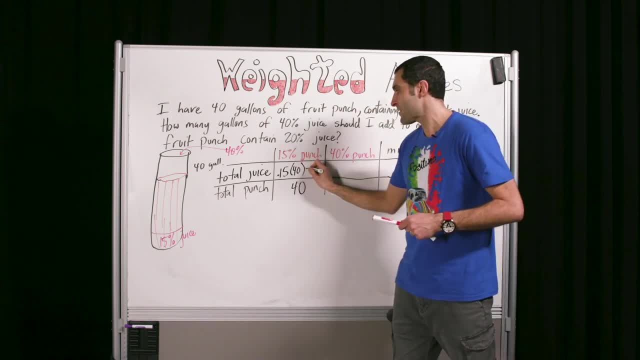 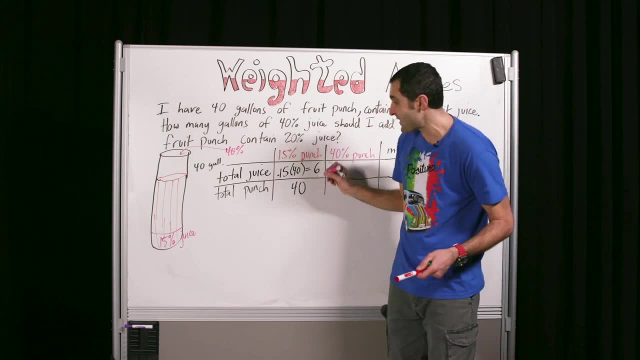 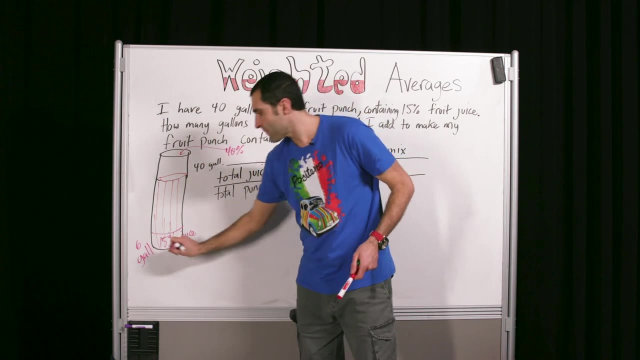 half of four is two. so four and two together that makes six. So six is 15% of 40. So of the 40 gallons, six gallons is juice, Six gallons Out of the 40, okay gallons. 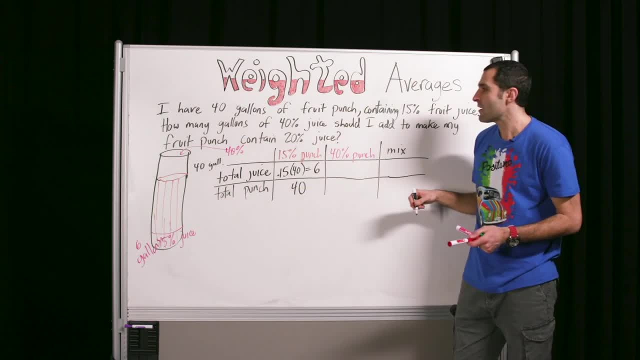 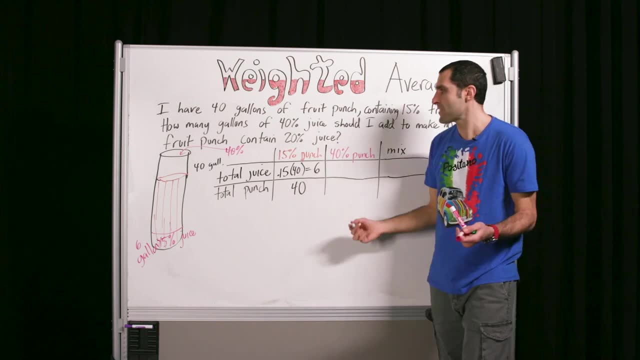 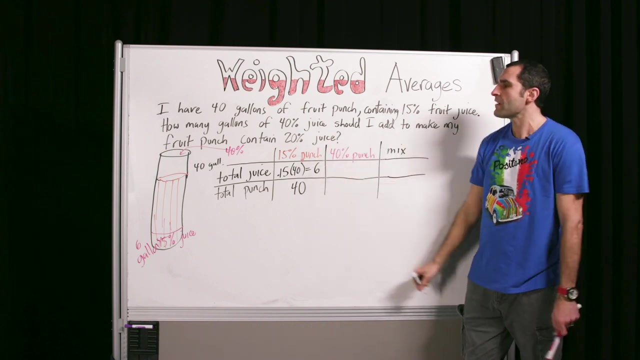 So far, so good. Then we put in the 40% punch. How many gallons of 40% punch? you know 40% juice in punch. you could say, should I add to make my thing a different concentration? Okay, how many gallons? 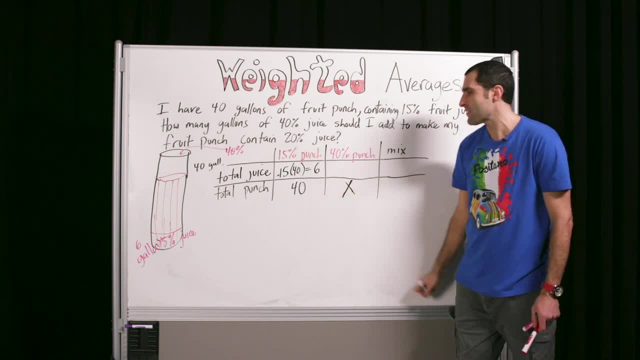 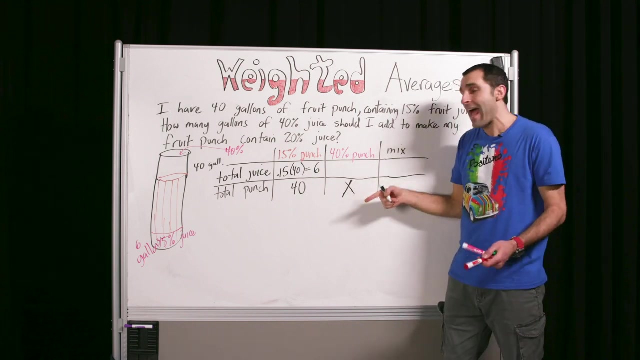 We don't know. We don't know how many gallons of this punch to add. However, we do know how much of it is juice. We know that, in this X amount of total punch that we're adding in, 40% of this, 40% of the gallons is actual juice. 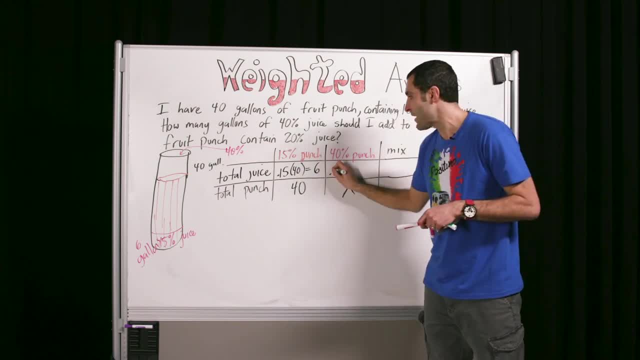 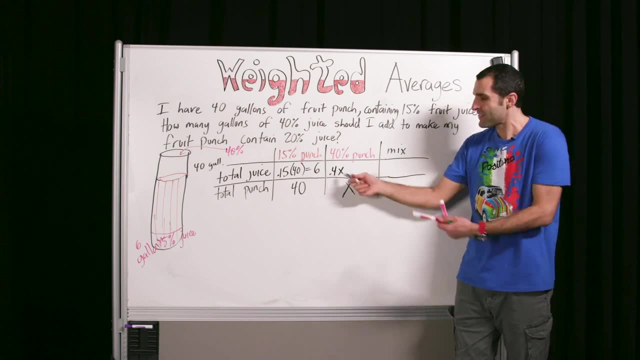 So, just like we did over here, we're gonna do 40.4 of X. All right, see that, Whatever this is, this is 40%, but we don't know what it is. but it's okay, We could still multiply them, okay. 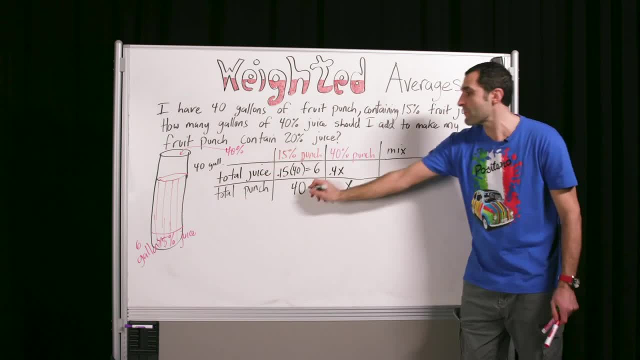 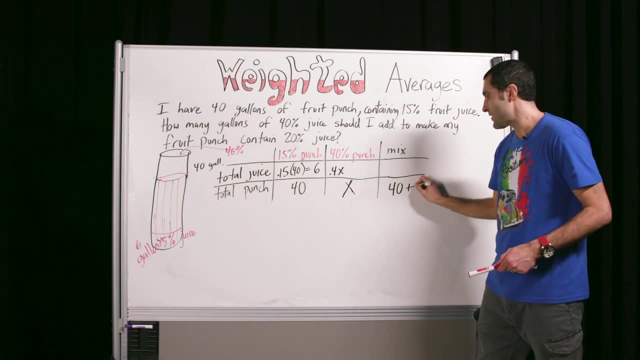 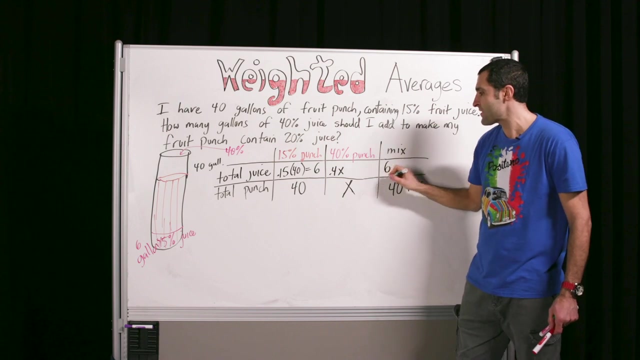 So we had some original amount and we added: We had some original amount and we added. So the total liquid in this container is 40 plus X. That's the total liquid, And the total juice is right here. We started with six gallons of juice. 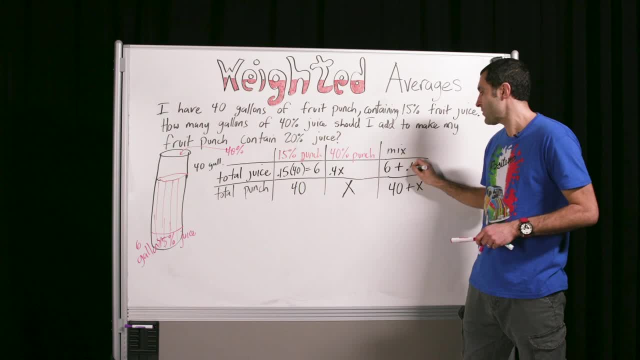 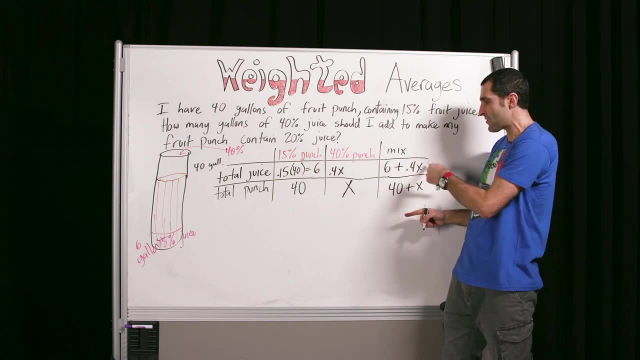 and we added- it's weird, but it's true- .4X gallons of juice. So we added six to this too. That's the total amount of juice, pure juice- And this is the total amount of liquid. So this is the ratio of the new mix. 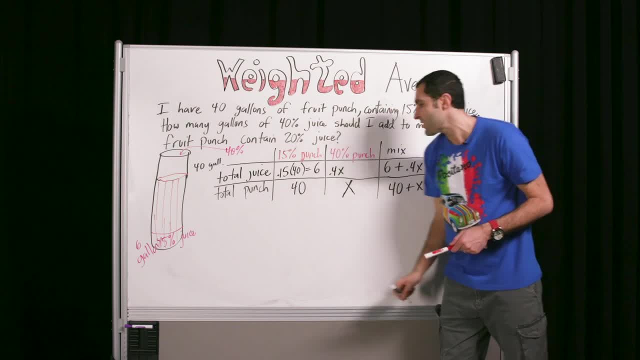 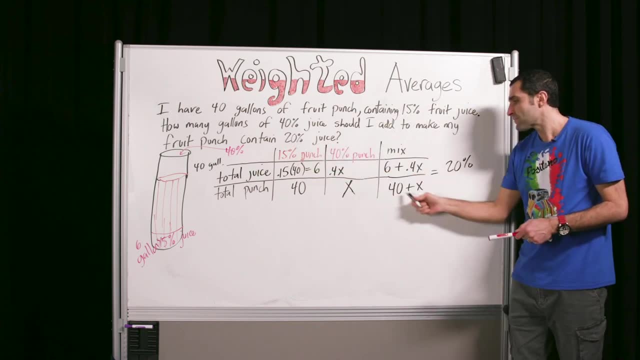 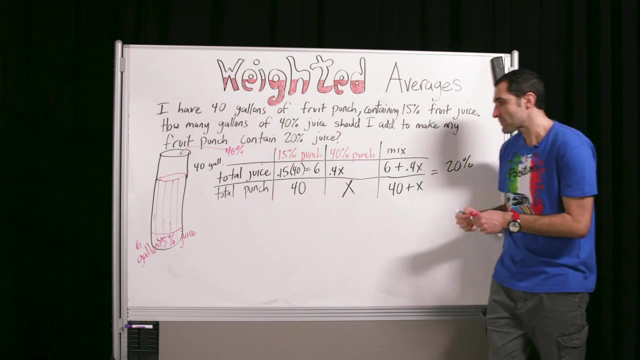 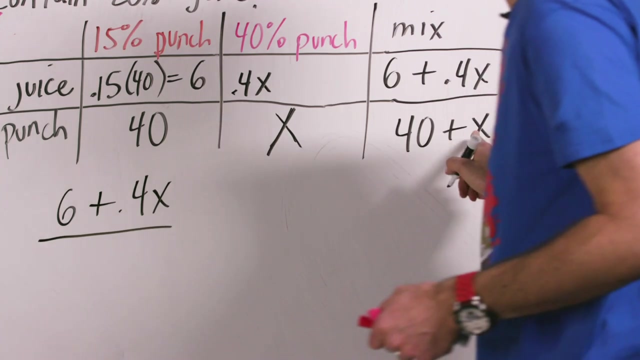 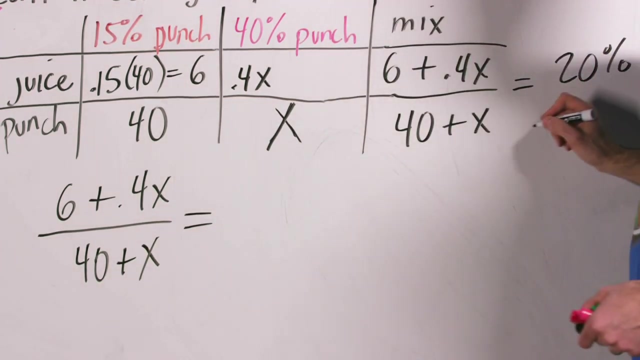 This ratio of juice to bottom, Juice to punch, must be 20%. All right, and now we can create an equation, right? This is the part where it pays off. So let's do our ratio: Juice to punch equals 20%. 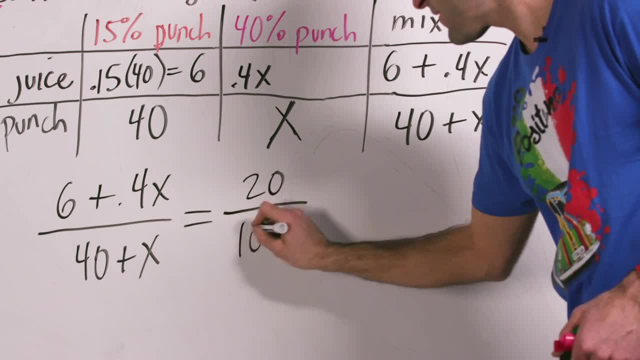 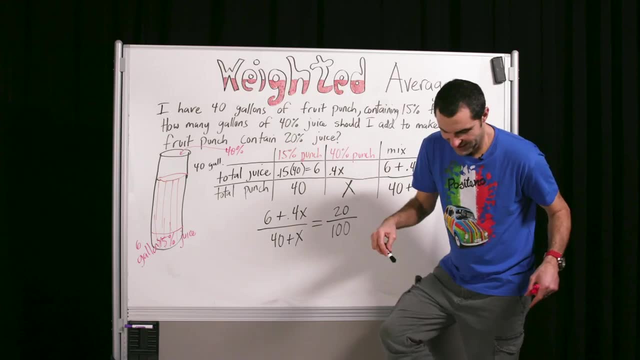 20% means over 100.. It's gotten real. I'm going to take my shoes off. Let's do this. It's getting real now. Here we go. I'm going to take this on comfortably. It's like we're in the family room now. 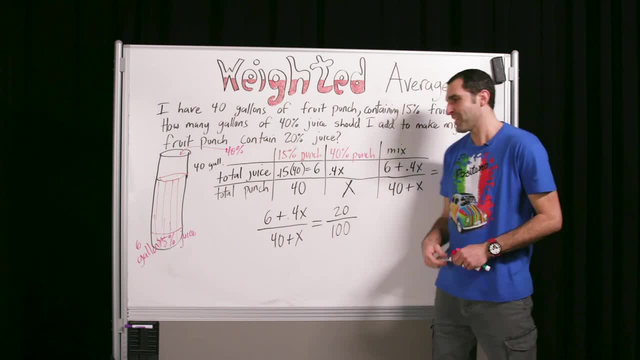 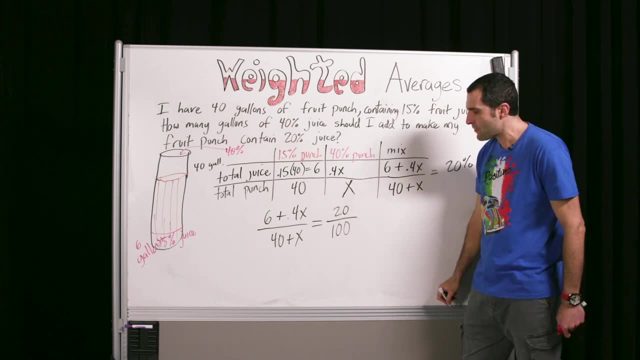 Let's do this. This is a home environment. Here we go. Let's do it: 20 over 100.. Good, So we could simplify this. It's always good, Cross multiplication will help, But before we cross multiply, what we can do is we can simplify. 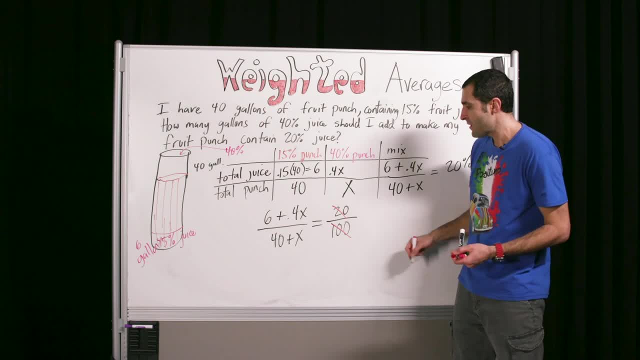 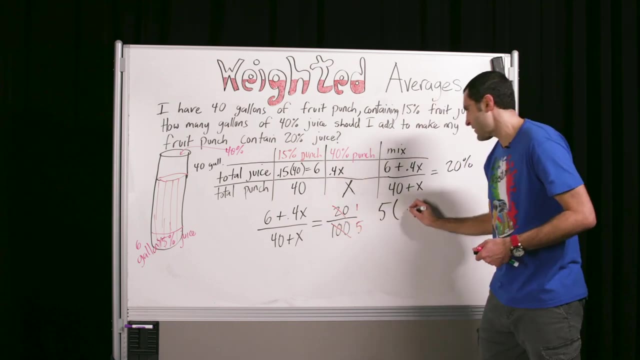 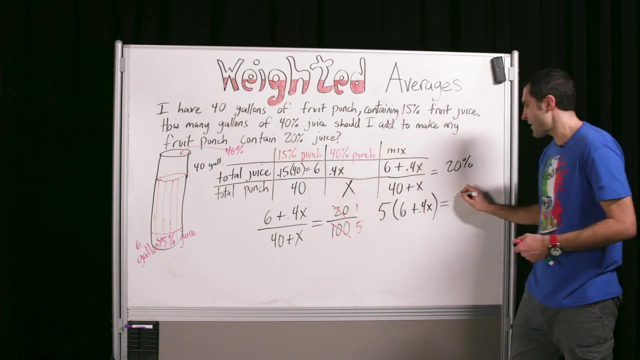 20 and 100 have a common factor of 20, and that's 1 over 5.. So now we can cross multiply. 5 hits this. Let's write it all out: 5 times 6 plus 0.4x equals 1 times 40 plus x. 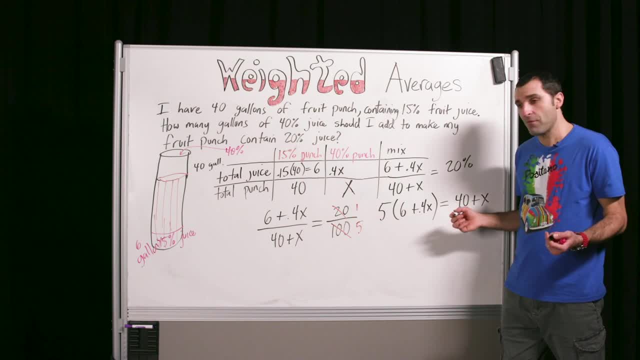 Good, There we go, And now we distribute and solve, Solving for x, 5 times 6,, 30.. Plus 0.4.. Times 5 is 2.. So it's 5 times 4, which is 20, and then move the decimal. 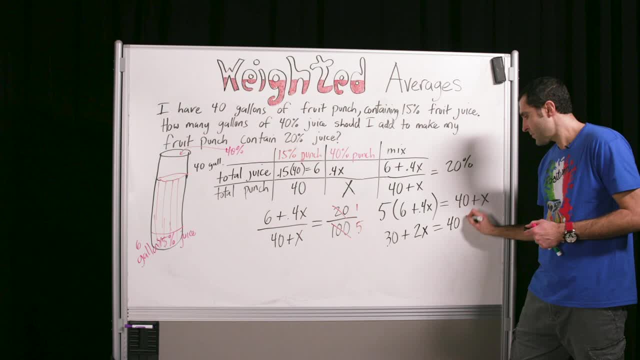 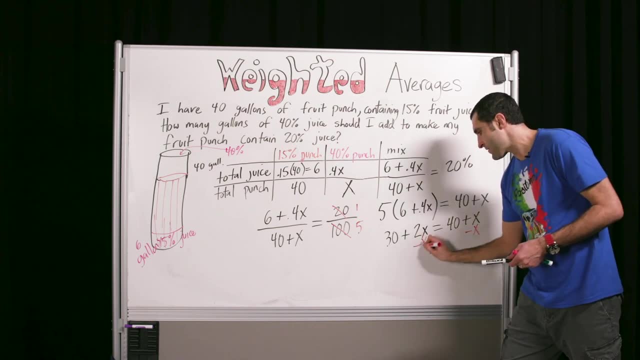 So that's: 2x equals 40 plus x. All right, I'm moving stuff around. I'm going to solve for x Minus x, both sides, Minus x, both sides. There it is, I'll bring the 30 over. 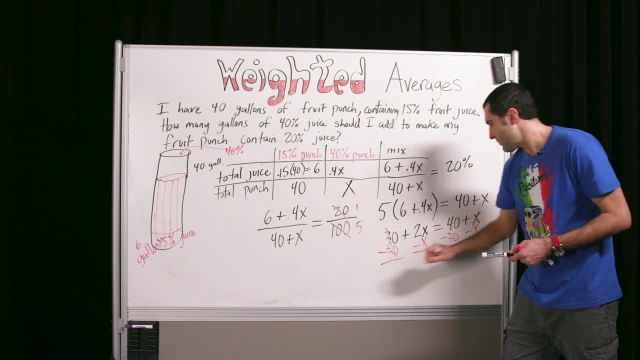 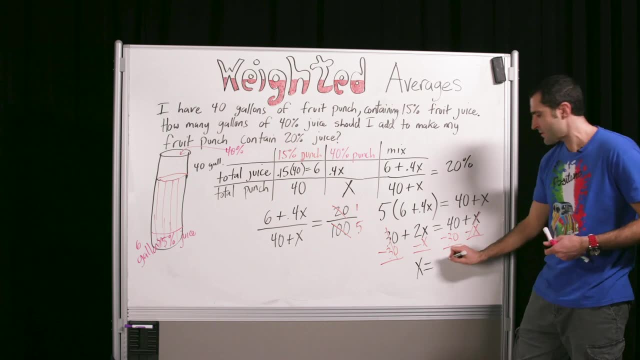 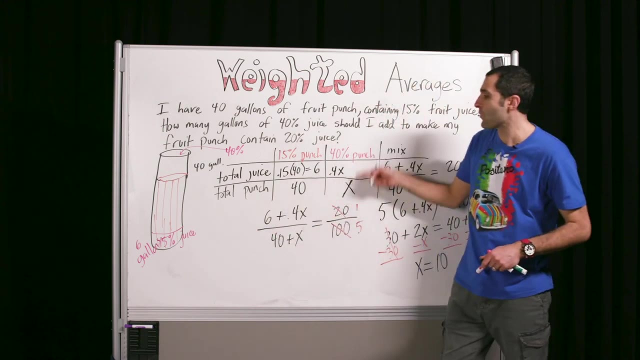 There, I need some of that juice right now. Here we go, Boom. So now we got 2x minus x is x Equals. there it is 10.. What is x measuring The total amount of punch that we added the 40%. 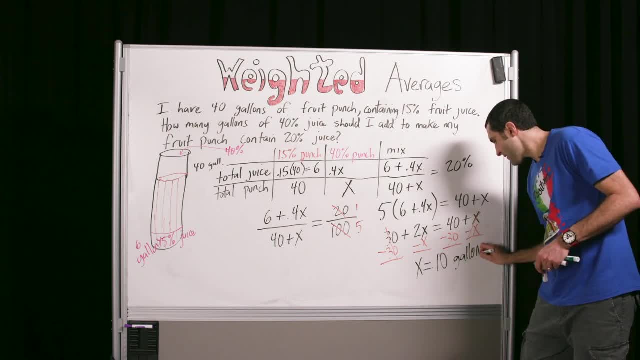 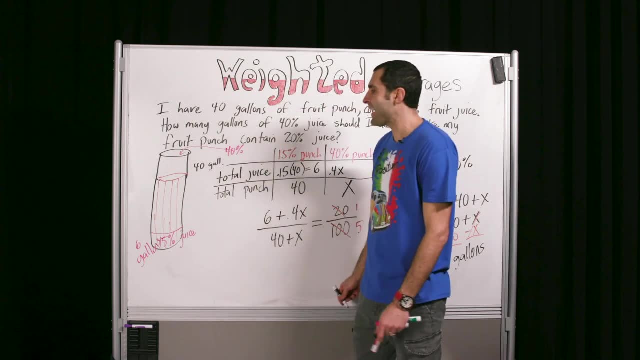 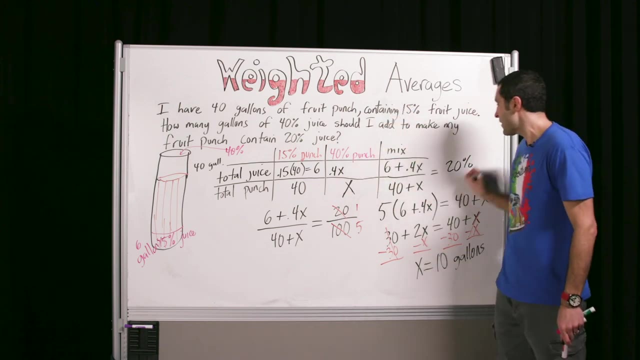 So this is we have to add. It's kind of fascinating If you had 40 gallons at 15% juice concentrate. if you added 10 gallons of 40% concentrate, the end result would be 20% concentrate. All right, 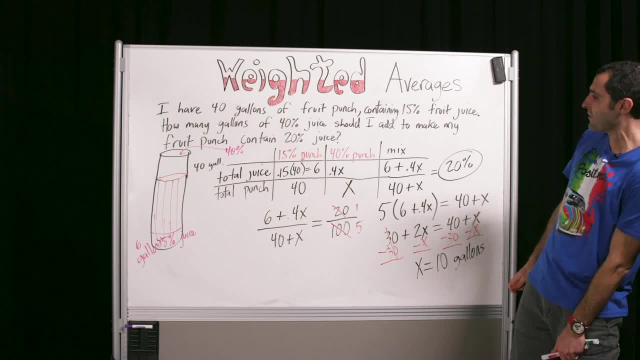 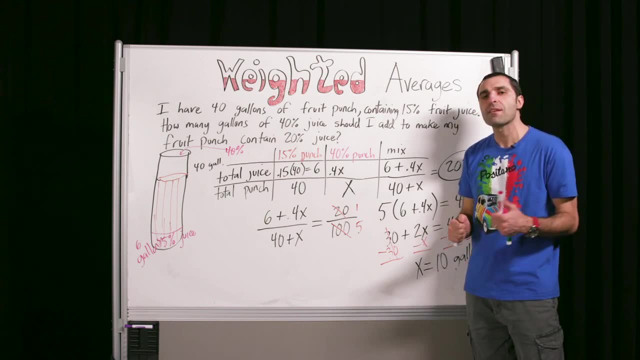 So that's the juice problem. Looking at it together, wow, It's hardcore. I really don't blame people for having a little hesitation for doing this stuff, But I'm just trying to introduce it in ways to remove some of that hesitation. 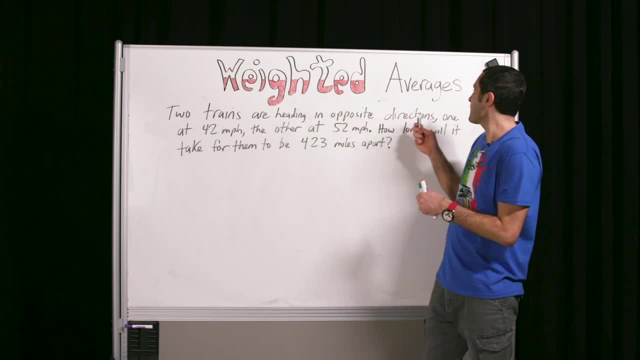 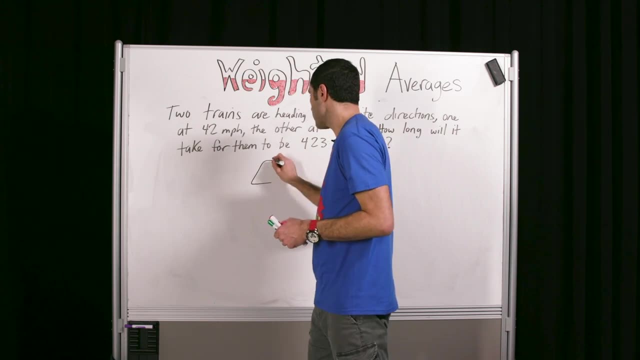 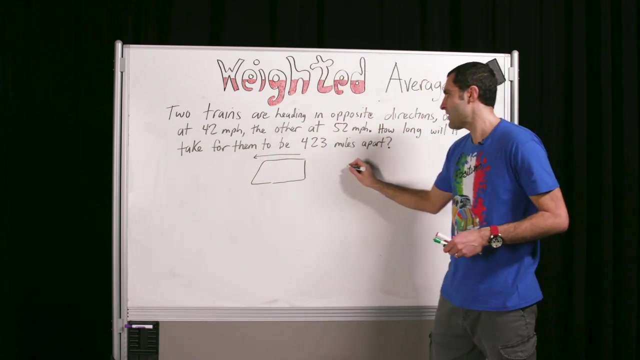 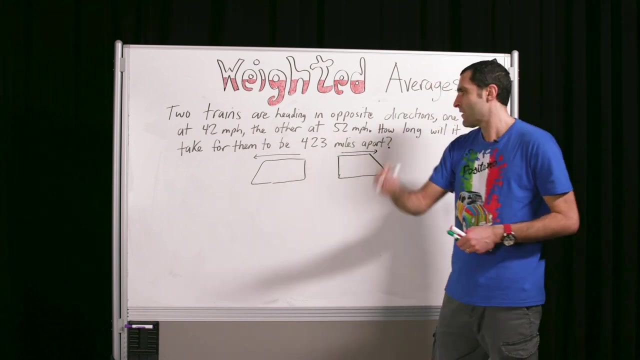 Next problem: Two trains are heading in opposite directions. Let's draw them. Let's draw the two trains. There we go. One is going, This is a short train, It's all good. And then we got. At least they sound the same. 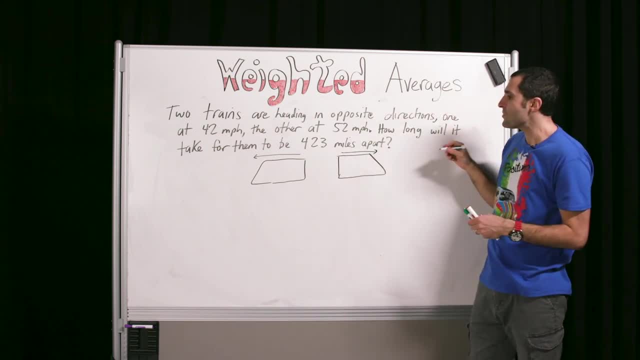 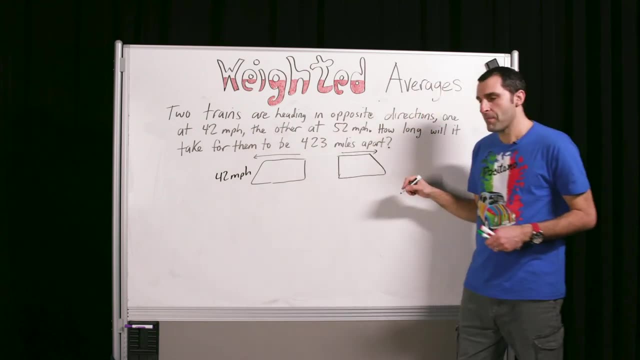 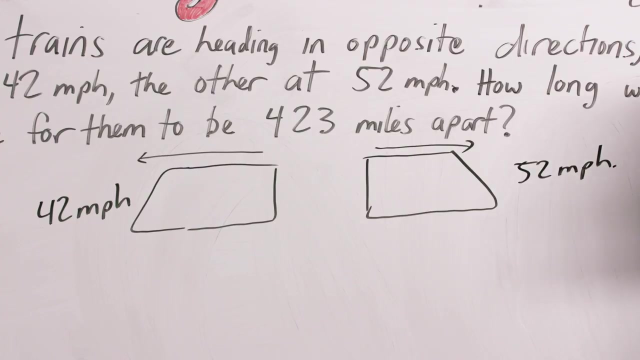 Heading in opposite directions. One is going 42 miles per hour, Put it. One is going 52 miles per hour Faster, Okay, Okay, How long will it take for them to be 423 miles apart from each other? Okay, 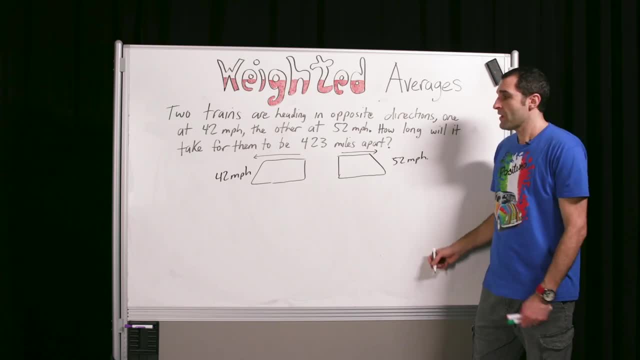 You could reason this out Or we could create an equation. The way to create the equation, a really good method for a lot, a lot of word problems, is creating a table or creating a chart here, Just like we did in the last problem. 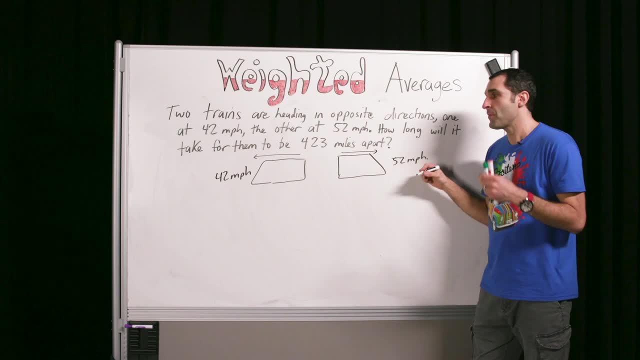 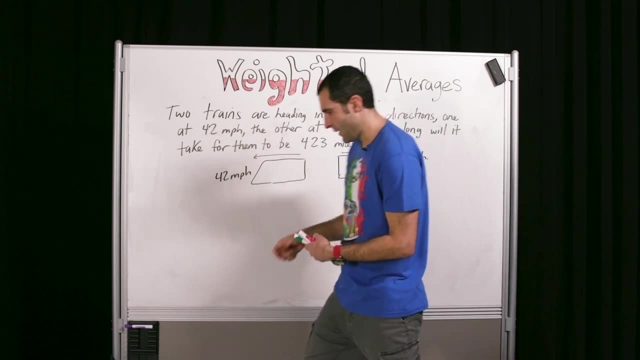 With distance and time and rate problems, we have the ironclad physics formula Which is- let's put it down here, Maybe in like perps- Actually I'll put it in black. The formula goes: rate times, time equals distance. 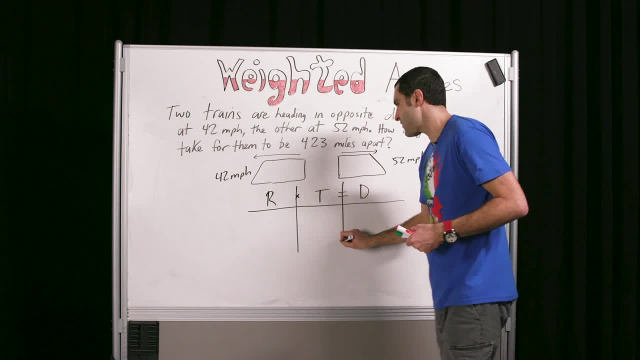 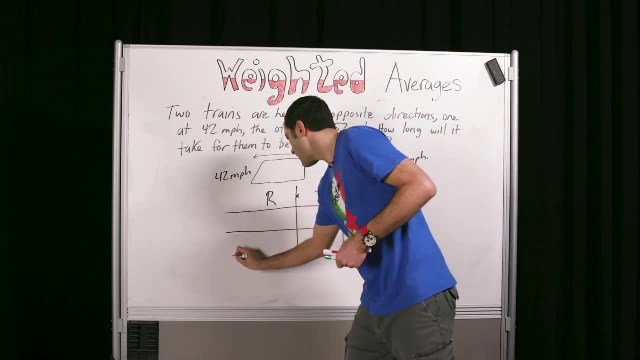 Right, We talked about not taking formulas wholesale. We don't want to lead with the formula. Never like, never start with the formula outright. You know it's not inspiring. Only time you should like have formula first is Okay, Okay. 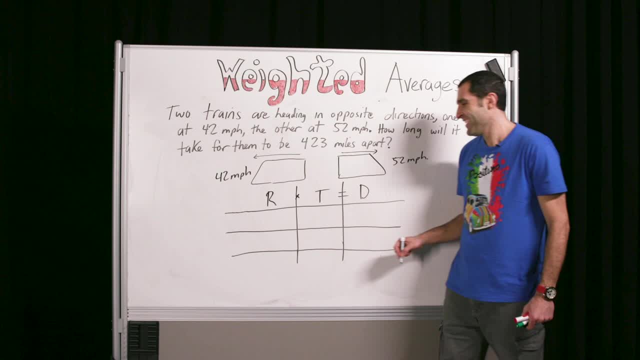 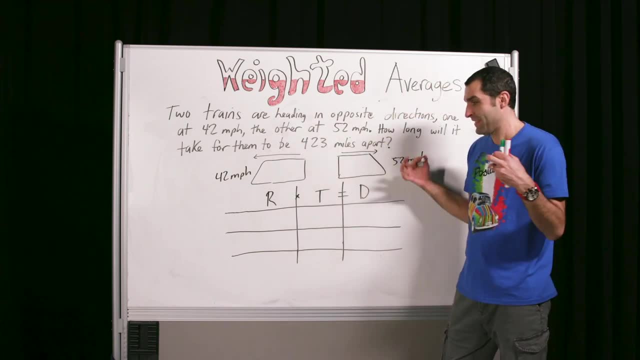 All right Feeling, I don't know- Feeding a baby. I'm waiting to eat that. But otherwise don't don't live with formulas: Rate times. time equals distance, You know it, I know it. If you're going like 60 miles per hour, 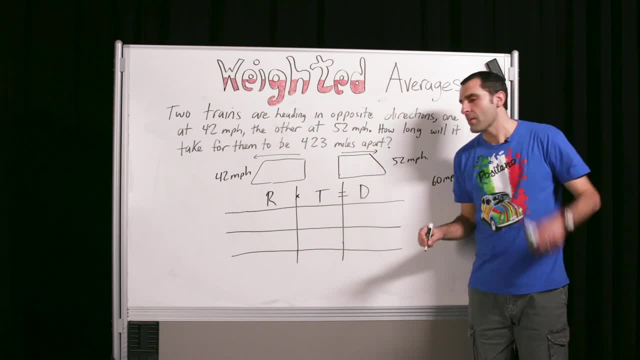 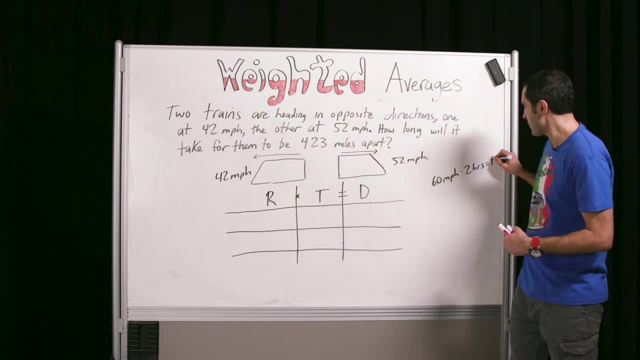 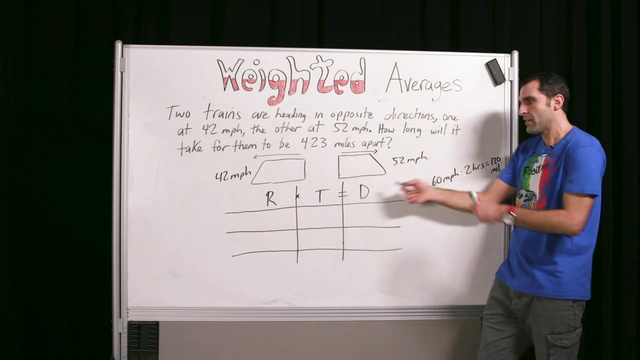 For two hours, Right, Immediately, you know. Oh, 60 miles per hour, Hour One, Hour Two. I went two of these sixties is 120 miles, So 50, which again 60, which Bada, bing, bada boom. You just did that Rate times time equals distance. So that's why. 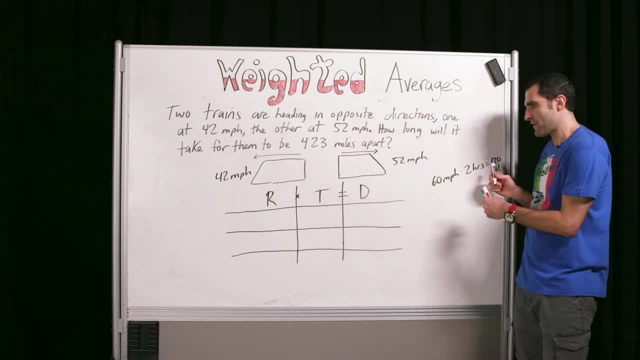 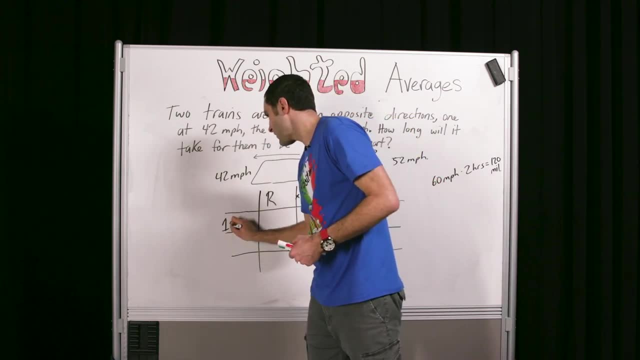 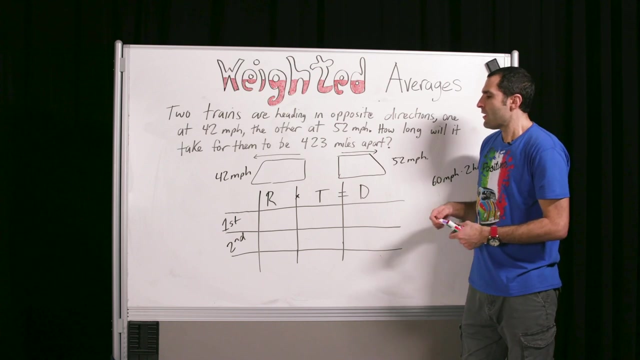 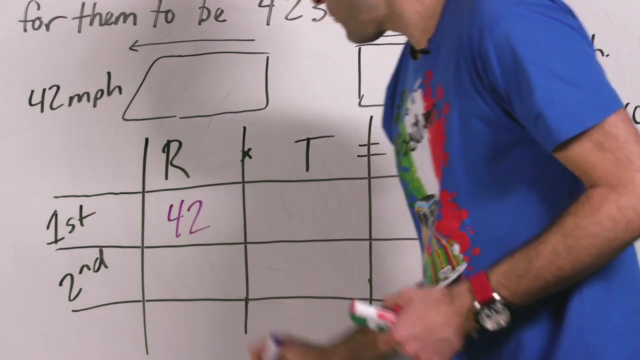 we're employing this formula: All right, Rate times. time equals distance, So let's do it. We have the first train and the second train. Now I'll pick a different color. Okay, Let's fill out what we know. Well, we know the rate of the first train: 42 miles per hour. Boom, We know the rate. 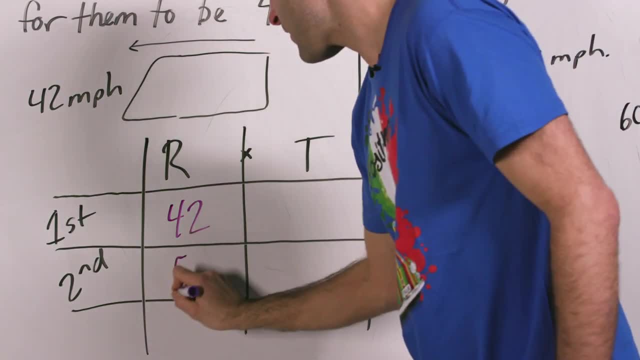 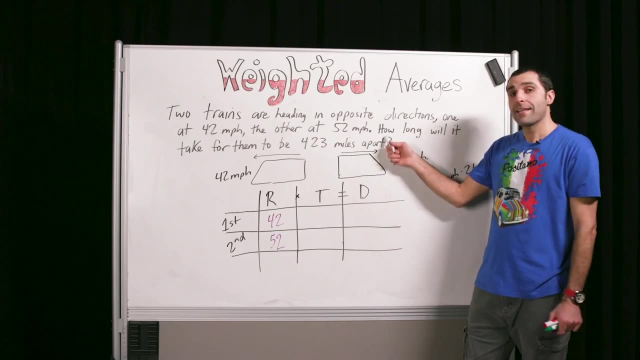 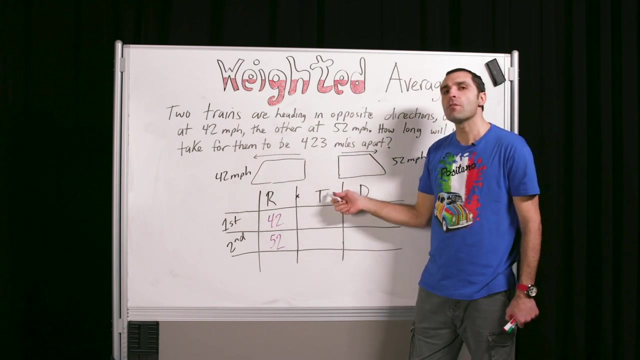 of the second train: 52 miles per hour. The time the first train goes, the time the second train goes. Check it out. How long will it take for them? Meaning how much time? Meaning we don't know this. The question is: are they going the same way? Are they going the same way? 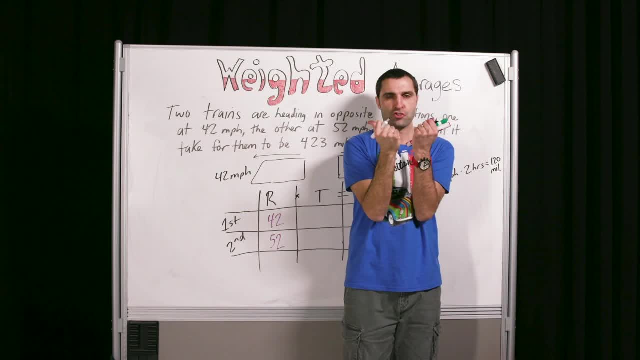 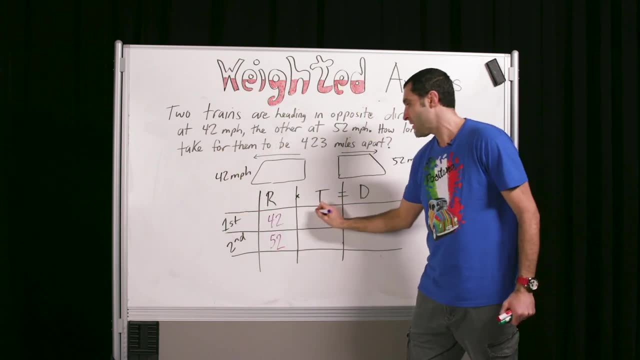 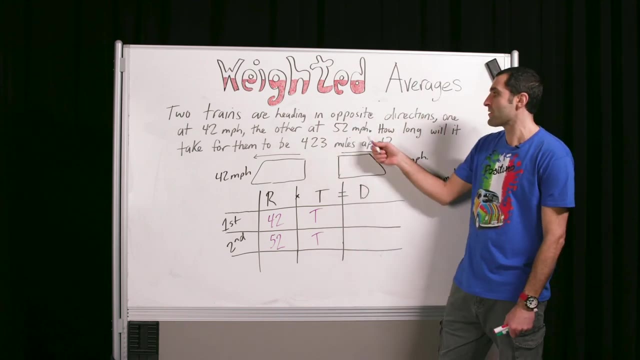 Are they going the same amount of time? Think it in your mind Like they leave. Stop. Yes, they are going the same amount of time. So they're going time and time. This will probably be measured in hours, right, Because we're at miles per hour. miles per hour, So this: 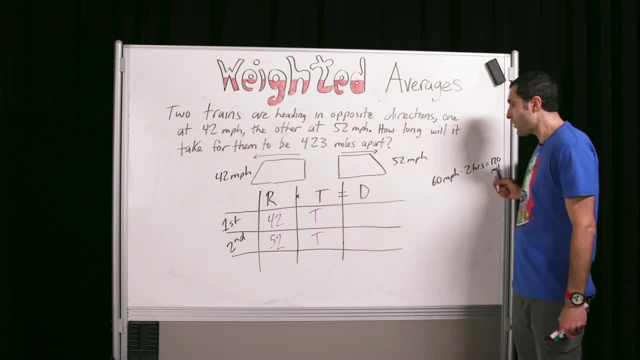 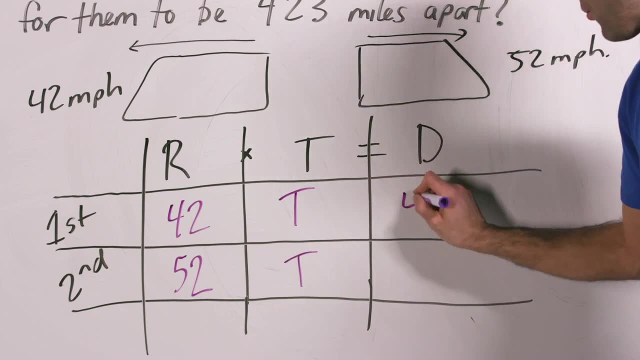 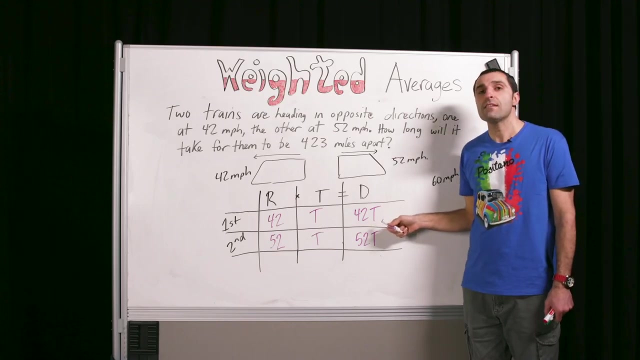 will be some matter of hours. Follow the formula: Rate times time is distance Rate times time is 42t. There it is 52t. Okay, So it turns out that the first train went 42t miles. That's a. 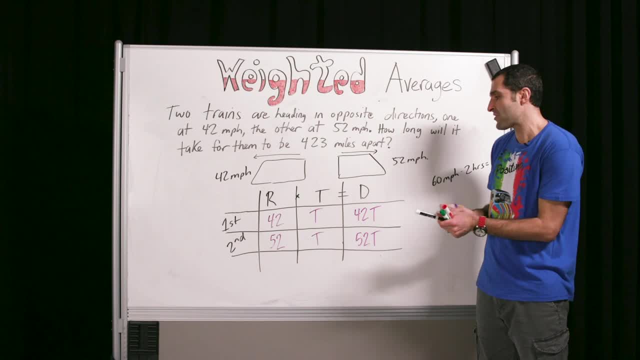 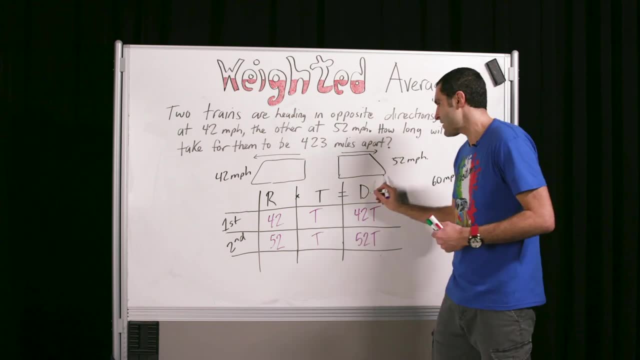 distance, That's a distance. It's a little strange to say, oh, how far did the train go? 42t. But it's really true, because if you don't know t, you just have to say 42t. So this is a distance. 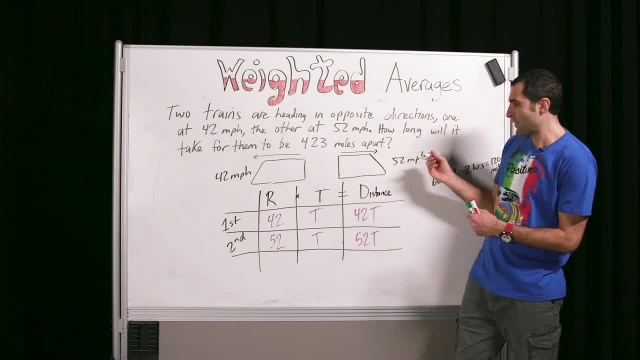 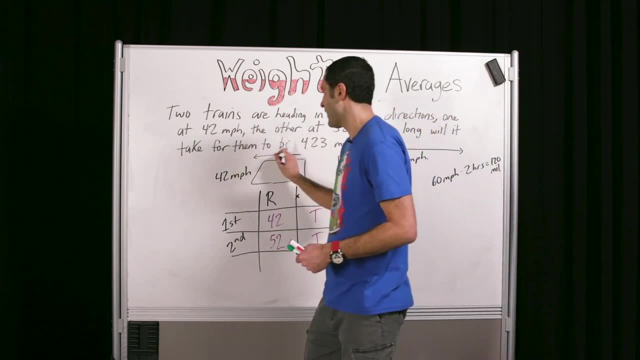 This distance is measured in miles, So in fact we could say it went la-la-la-la-la-la-la-la-la-la, This is well, that was the 52t, So we'll go over here La-la-la-la-la, like I was saying. 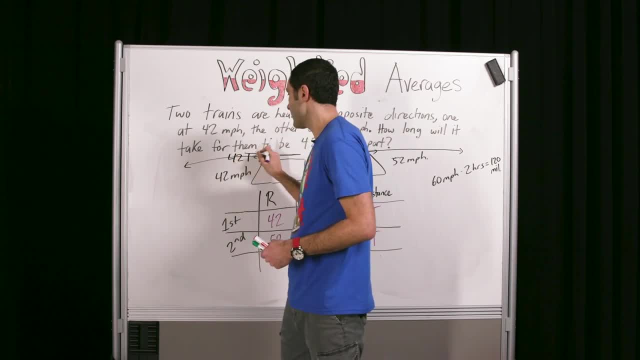 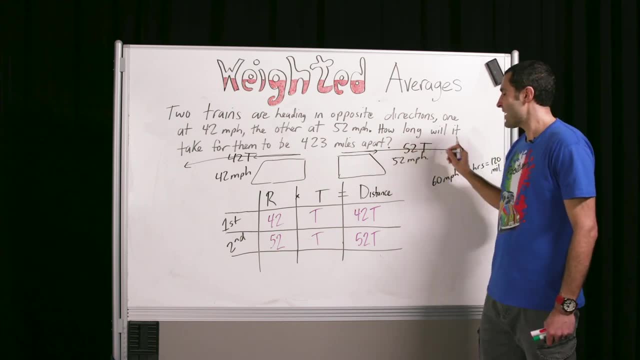 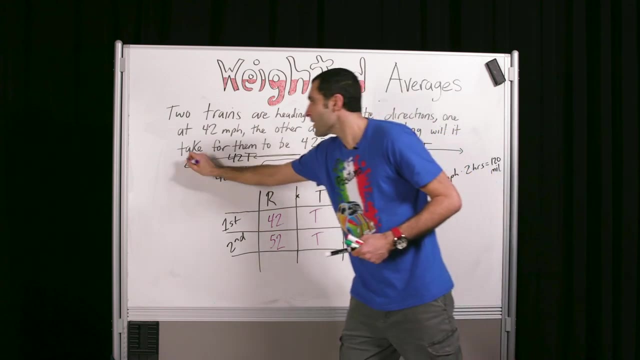 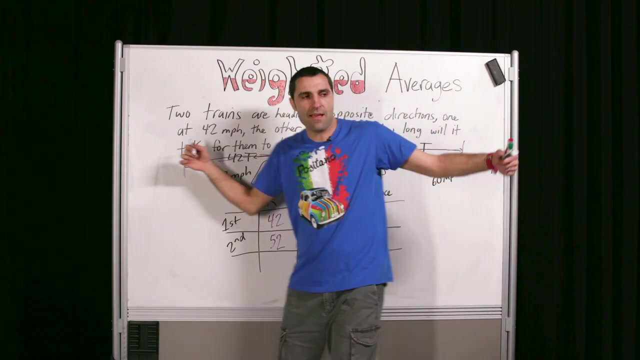 la-la-la-la-la: 42t, That's the distance that the first train went, 52t, That's the distance that the second train went, And it turns out that they should be 423 miles apart. This length between them, like at the ends between them, is 423.. So would it make. 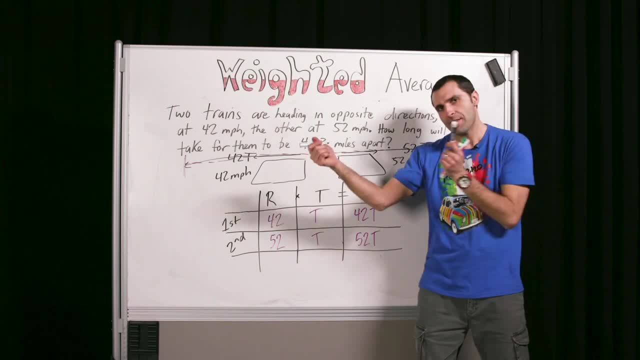 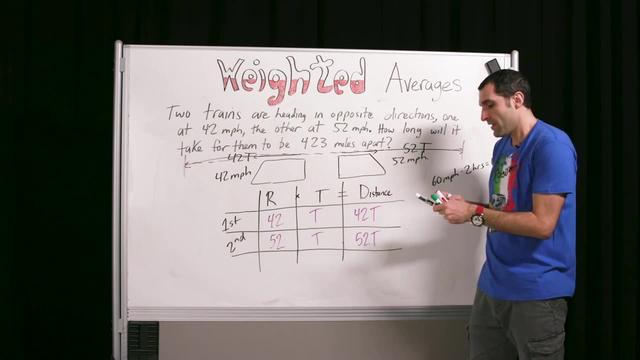 sense to you to add these two distances- one going this way, one going that way- and together they make 423? Because that's what we need to do. So I hope it does make sense. Let's do it. Let's do it. Here we go: 42t. I'll write it out. 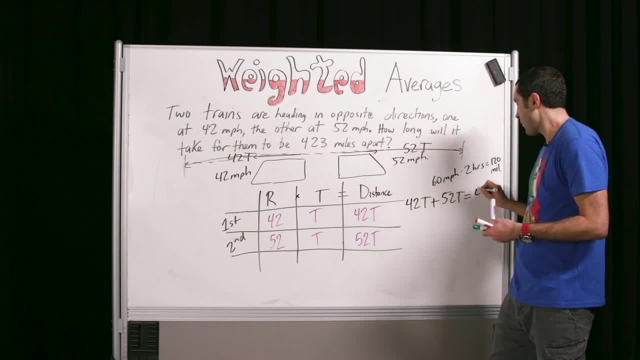 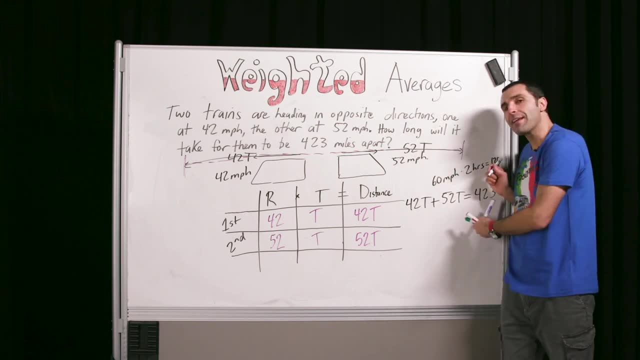 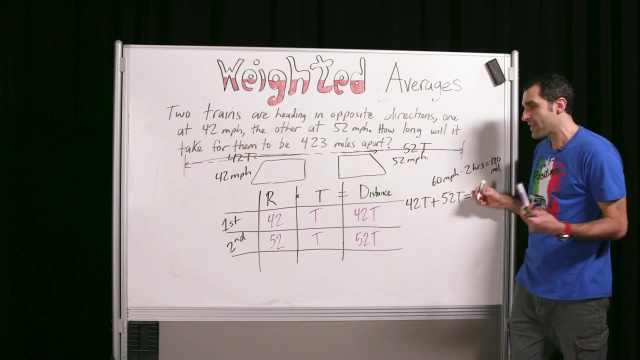 52t plus 52t equals 423.. Bravo, There it is. That's the equation, These two distances. Always make sure you create an equation that has the same units. This is a distance. This is a distance. This is a distance right. Never create an equation with distance and rate in it, For. 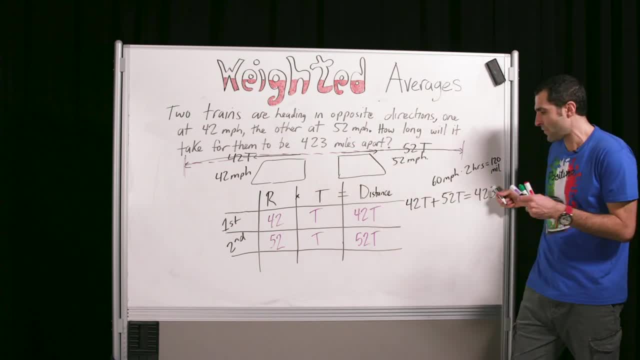 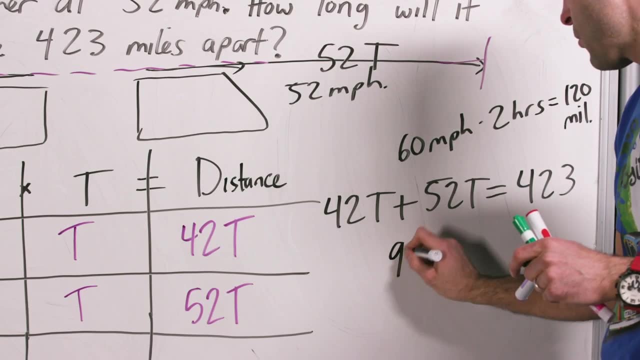 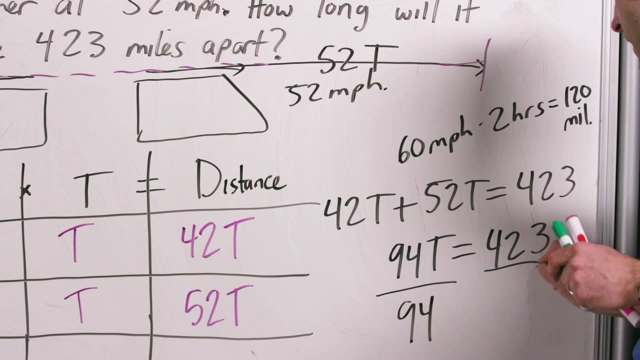 example, distance and time in it. You want to have an equation with one unit. Add them up. This is what is that? 94t equals 423.. Divide both sides by 94.. Divide both sides by 94.. Good, Yeah, 94.. Good, And let's. 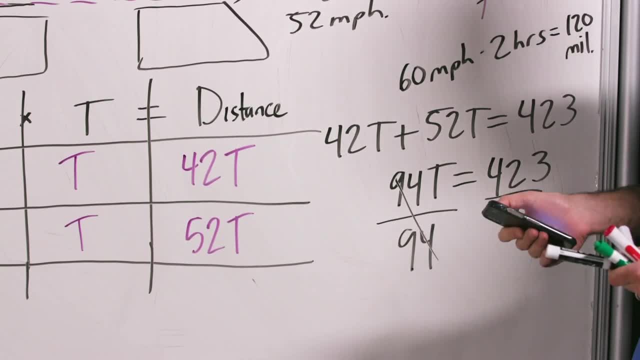 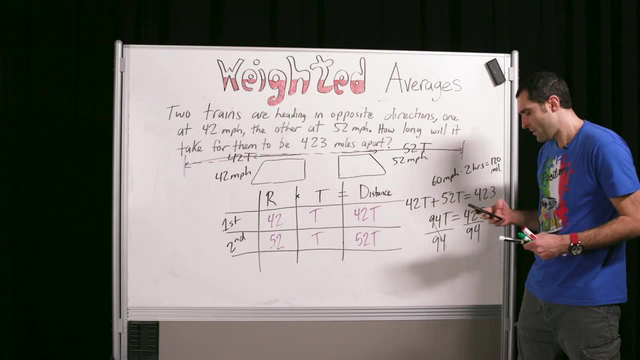 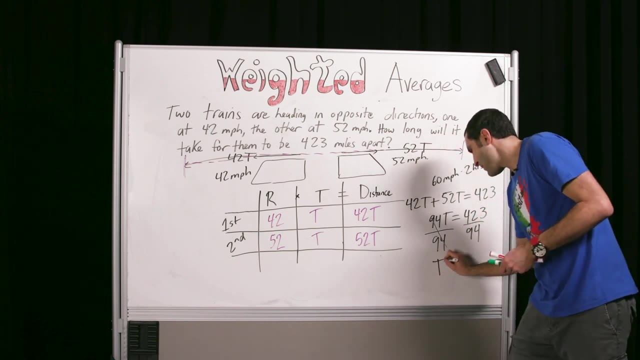 get the calc going. Unlock that, Here we go. 423 divided by 94.. 4.5. Said emphatically. And what are we measuring? 4.5.. What was t measuring? t is measuring time. Time is measured in. 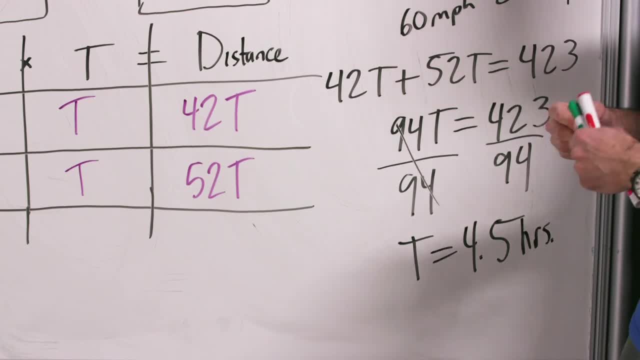 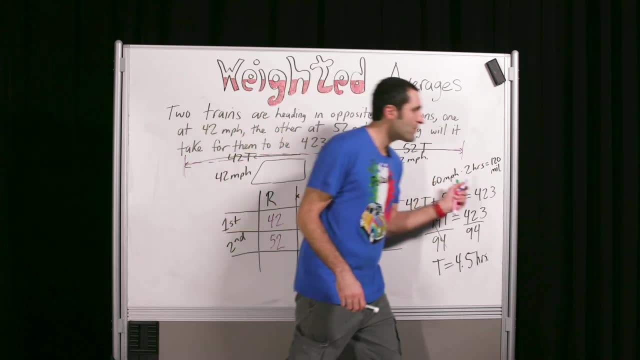 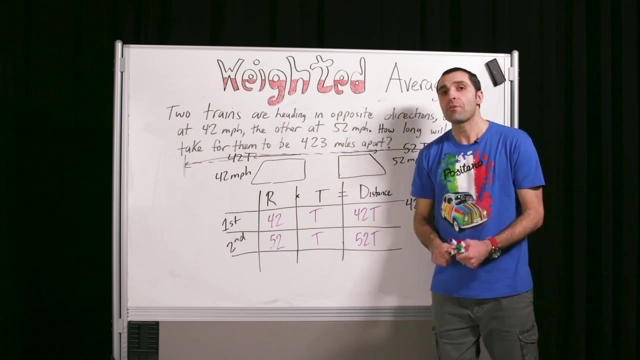 units of hours, So it's important to articulate it in a full sentence: If one train is going in one direction at 42 miles an hour, the other train going at 52 miles an hour, after four and a half hours they would be 423 miles apart. All right, It's been satisfying about it. 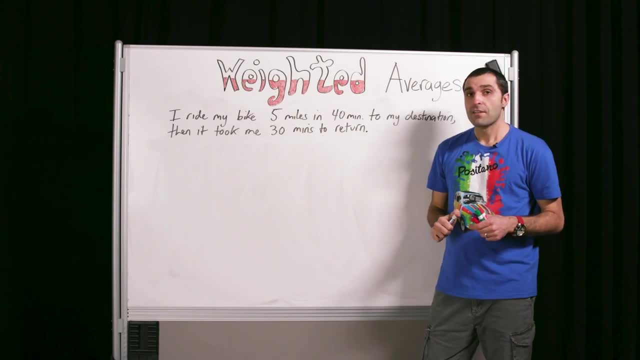 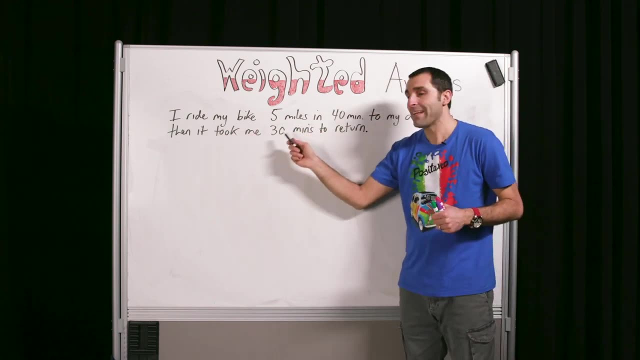 All right, Let's move on. Two to go- Good, All right. Next problem: So suppose I ride my bike for five miles and it takes 40 minutes to get to my destination, And then it takes me 30 minutes to. 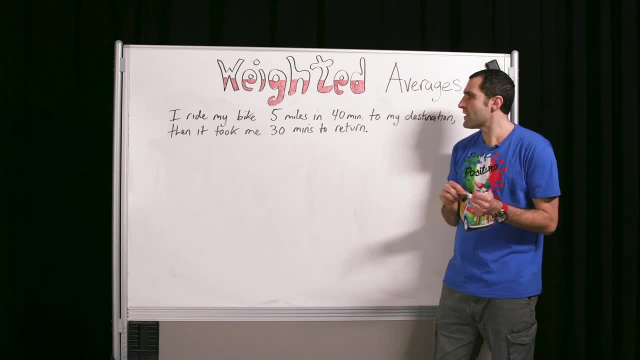 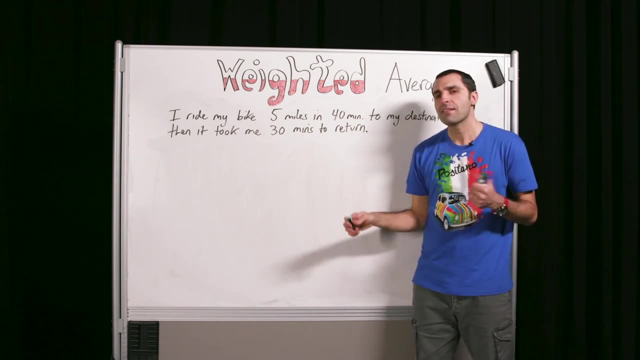 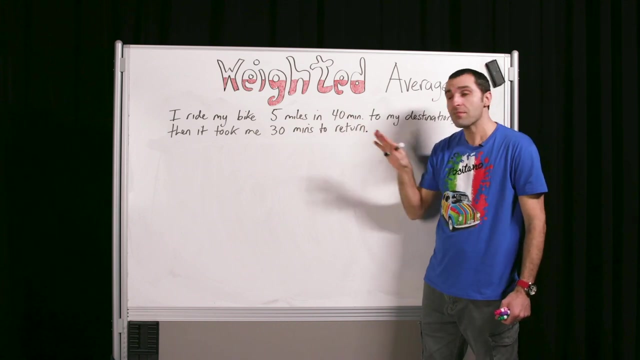 get back. So a couple things. First of all, let's see how that makes sense. If you've ever ridden a bike before, if it takes you 40 minutes to get somewhere and 30 minutes to get back, most likely it's because I'm like chugging it hard. It's probably because on the way there it's uphill. 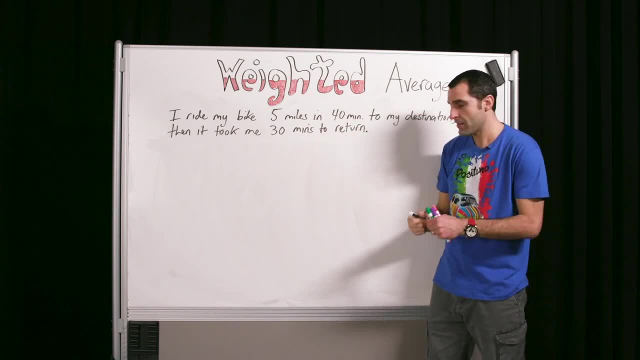 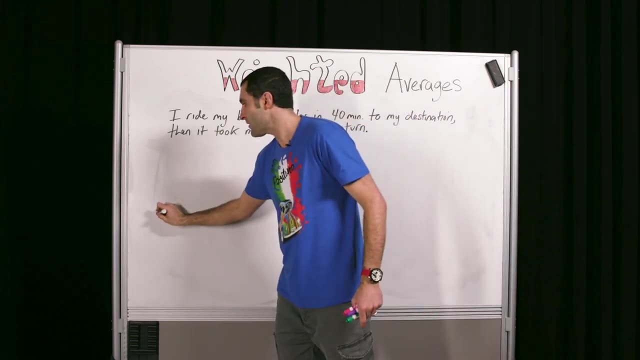 took me longer On the way back. it's downhill right, So it took me less time. It's still five miles, though, Keep that in mind. So let's say I'm here, I start here, go up. This is. 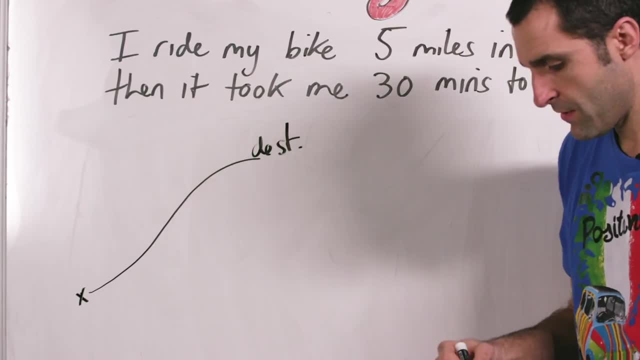 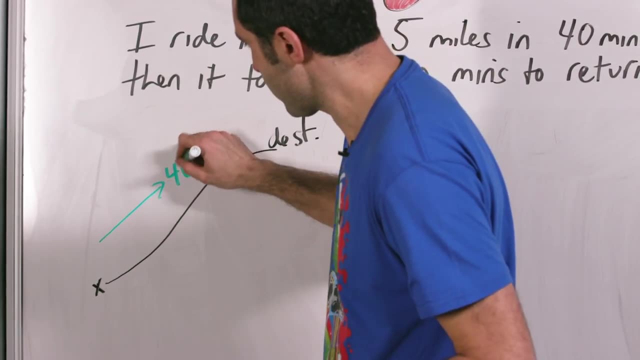 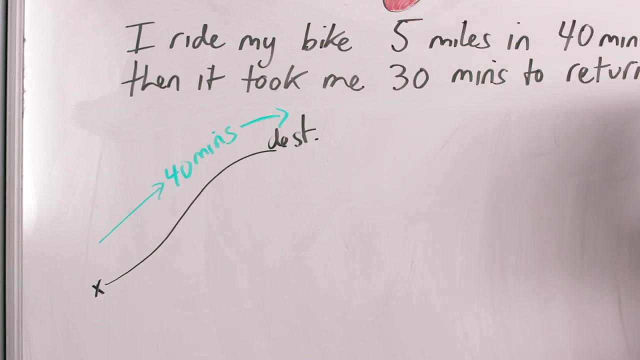 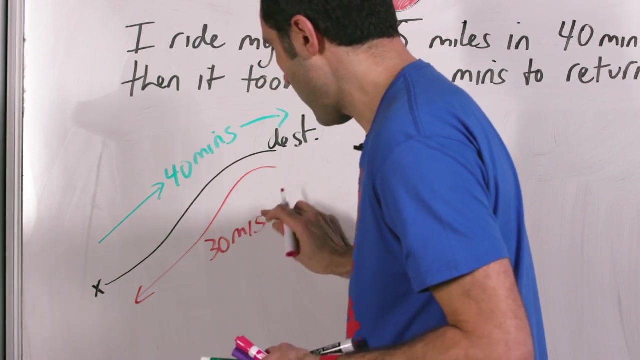 the destination It took me. let's go there in green. This was 40 mins. I'm going to go five miles, Five miles, And then it took me 30 minutes to get back. Kind of interesting Back 30 minutes, All right. So that's the first thing to keep in mind Sometimes, the time it takes to go. 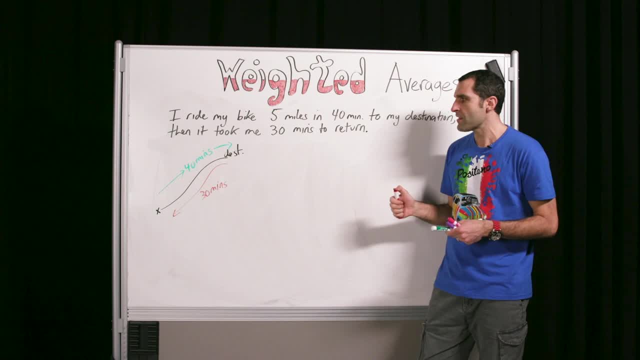 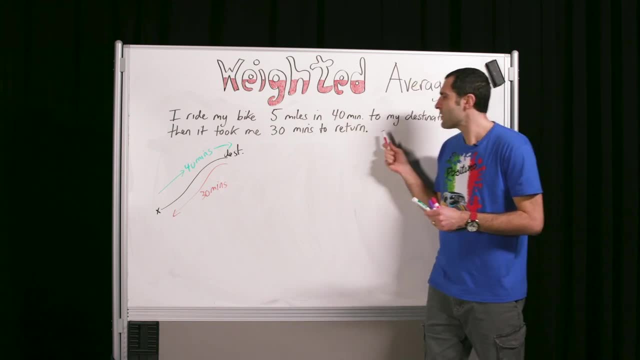 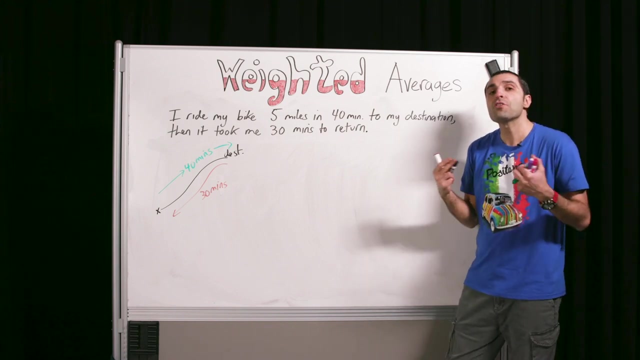 there and back are different, based on hills, in this case. Common sense, Or it's a common sense assumption, right? I didn't ask a question yet I did that on purpose. What could I ask? What could I ask? There's a huge sense of empowerment in figuring out what you could ask. 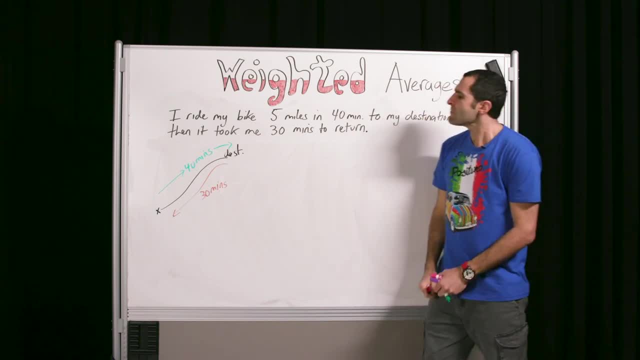 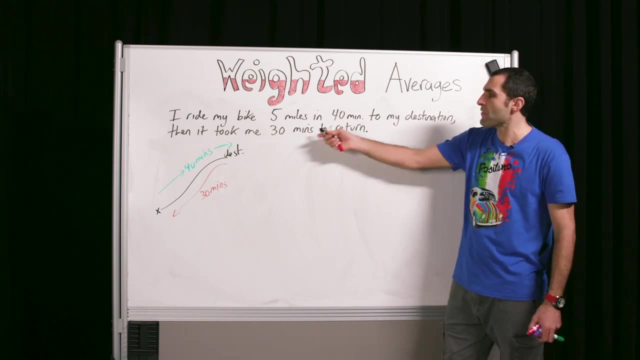 because it's like, then you need to know, like, well, what am I missing? Let's see, I could ask like: or should I ask the total time? Not really No, because I know it's 40 minutes there and 30. 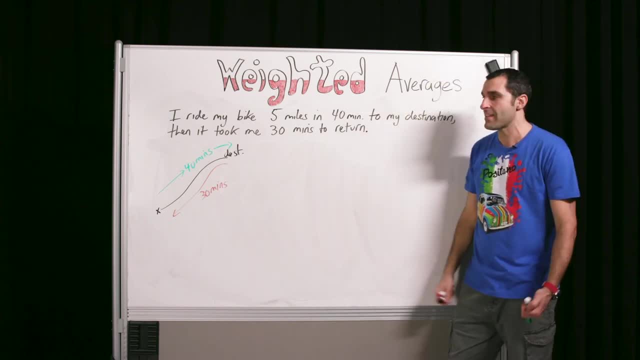 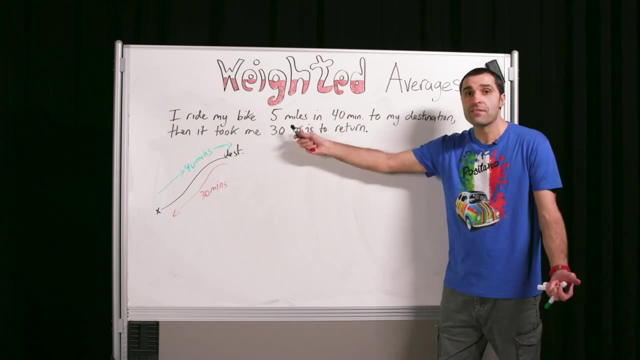 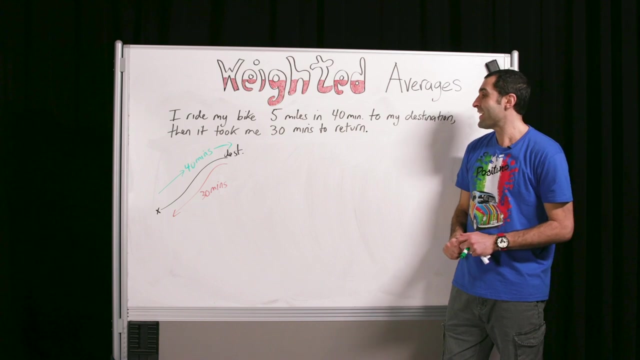 minutes back, 70 minutes round trip. So I already know the total time. I don't need to ask that Total distance traveled. I know that as well. Five miles there, five miles that back. That's 10 miles Round trip. So what could I ask? A hint: if you don't have that question in your mind, has to do. 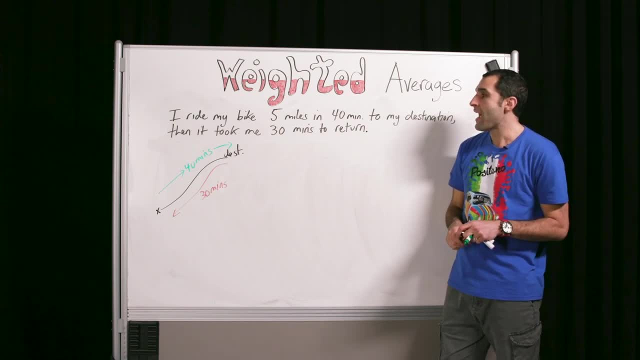 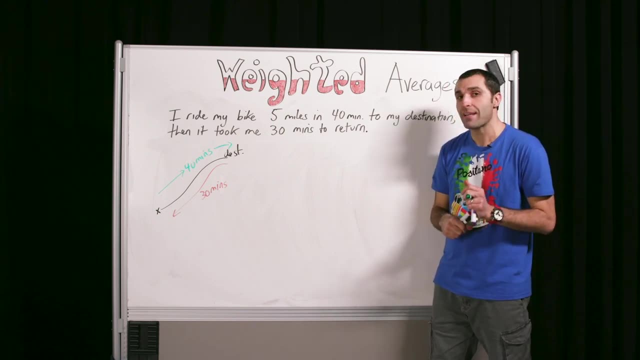 with my speed. Okay, So I could possibly calculate my speed there And I could possibly calculate my speed back. So we're going to do that. I don't know my speed there And I don't know my speed back. More importantly, since this is about averages, is what my average speed was. 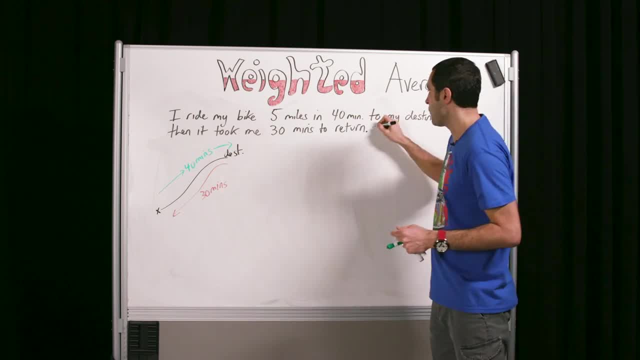 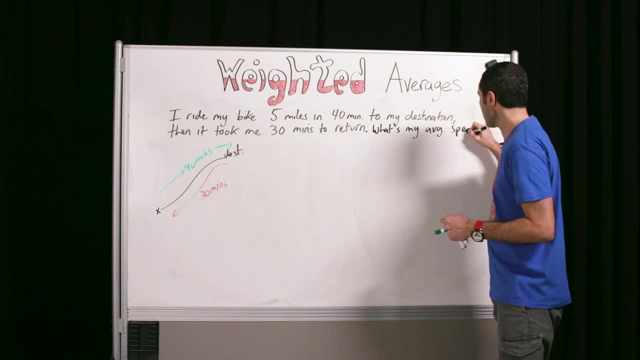 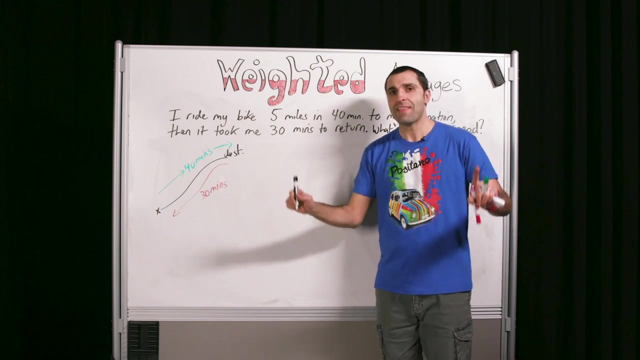 And this is where it gets really challenging- What's my average speed? Because I'll tell you right now: it's not the average of the two speeds. It's not the average of the two speeds, which is kind of so fascinating when I was learning this stuff and when I was 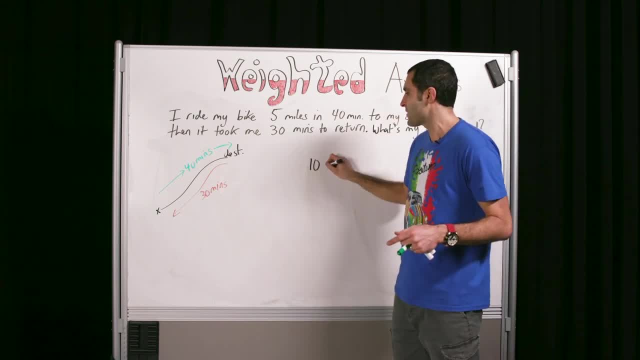 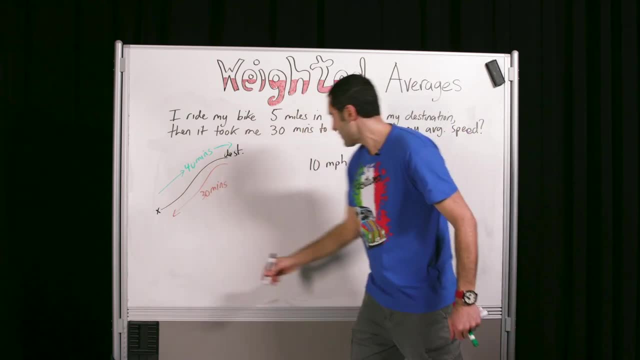 teaching it Like, if you think of it. let's just say hypothetically I was going 10 miles per hour back right, Because it was going downhill took me less time. And then let's say it took me 20 miles. 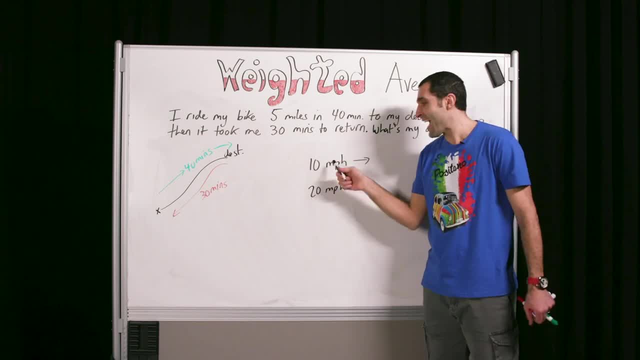 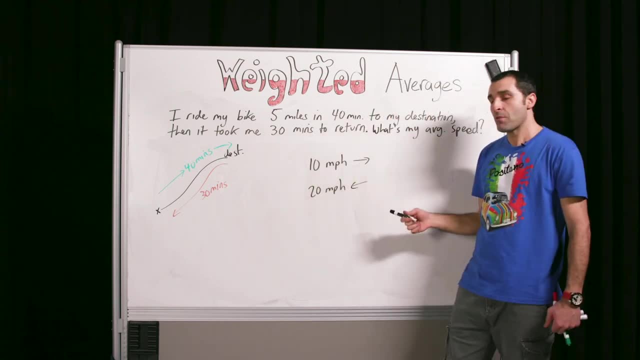 an hour back. The temptation is to average these. you know to say: yo oh, perfect, 10 miles an hour there, I was faster back, 20 miles an hour back. So the average is the middle of that, That's. 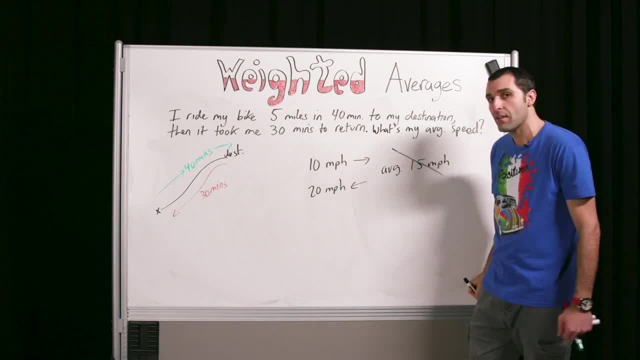 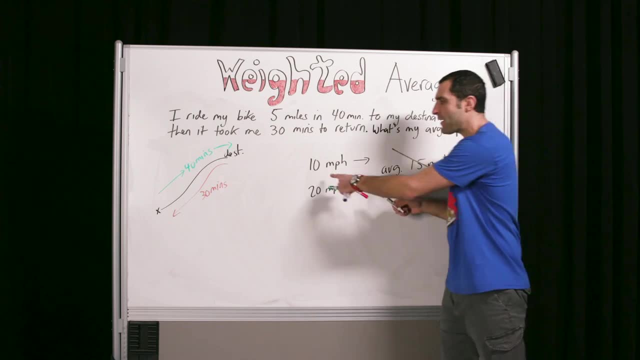 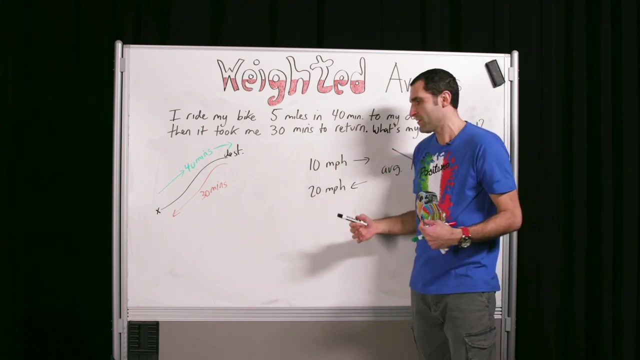 15 miles per hour. This is wrong Because I was riding for more time here. See what I mean. Like I went for more time slower. So in a sense, this is going to be weighted more. This is going to be weighted more for like, for longer It's chugging. It's chugging for 10 minutes more So on average. 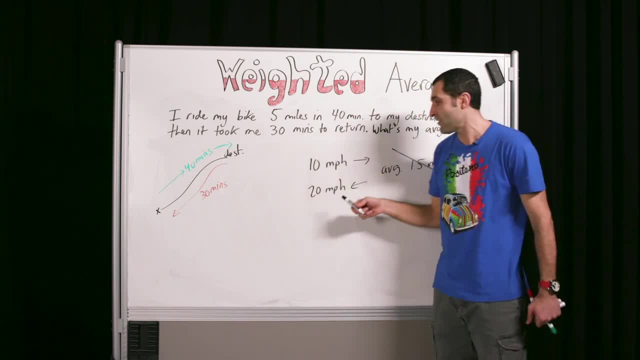 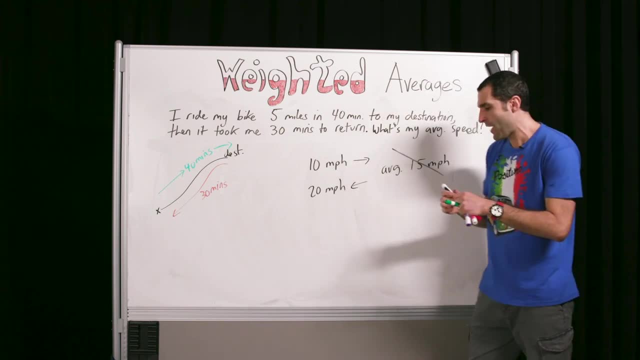 my speed will actually be lower compared to these two, So it wouldn't necessarily be 15, maybe like 14,, 13,, something like that. All right, So that's what I'm going to show you how this works. You have to sort of factor in the fact that we're 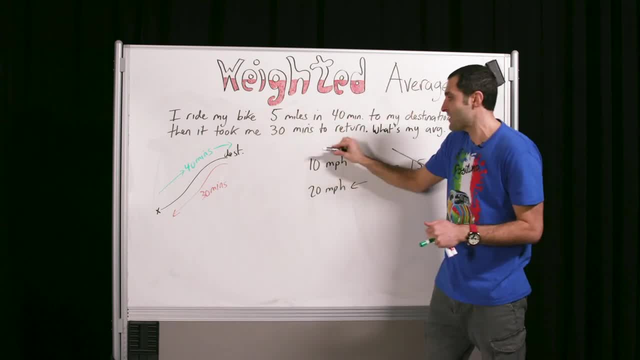 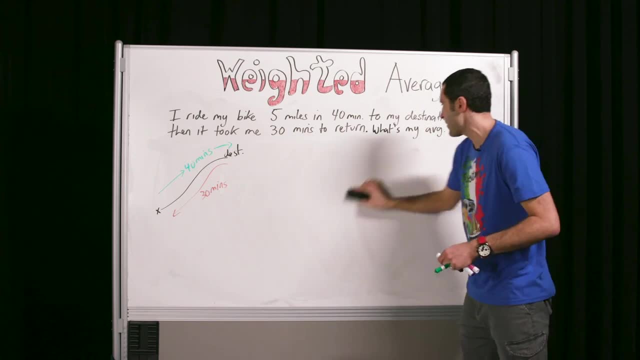 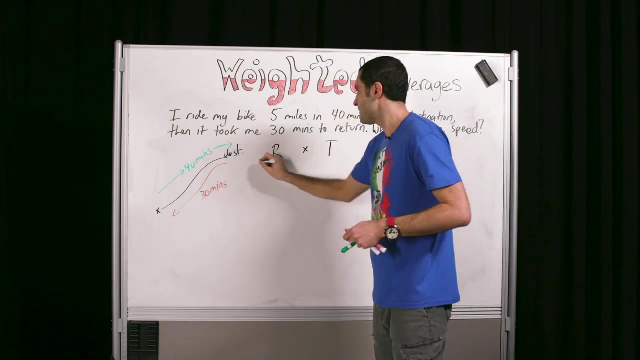 riding for longer in one direction, So it's not a straight traditional average. Okay, I hope that helped. So let's go ahead and do our distance equals rate times time process, starting with rate times. time equals D. All right, So we have there. 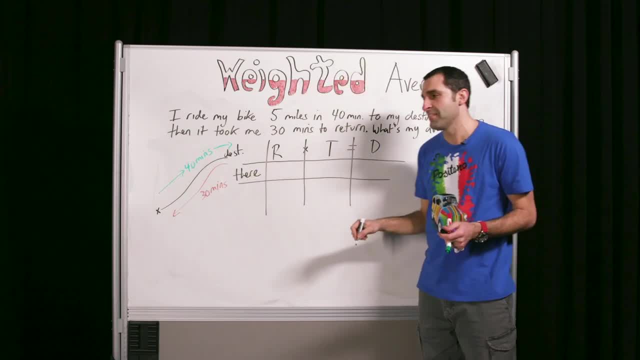 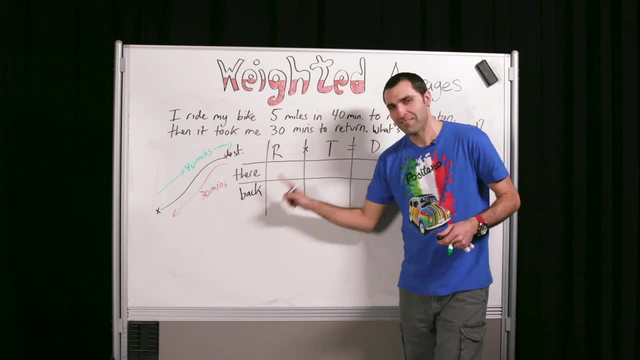 I should probably say there, there to you To calm you down: There, there, There, there and back. You'll be fine. I got your back There, there Got your back All right. So let's figure out what we know. The good thing about a chart is: 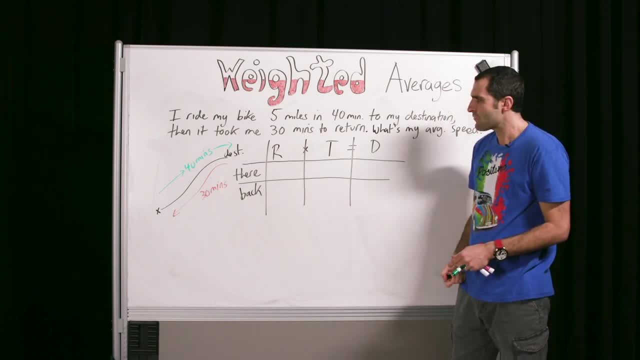 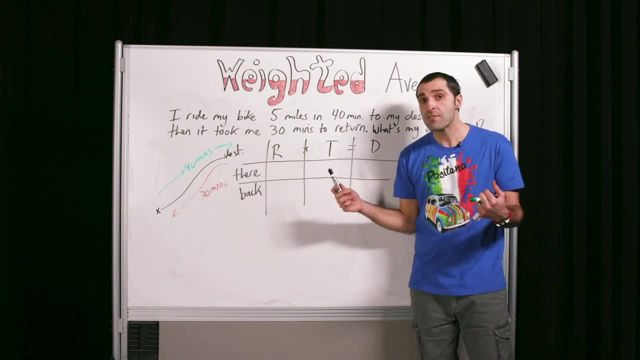 that you can just fill in one piece at a time. I don't really have the rate, but I do have the time. What I'd like to do is I like to put the time into hours, even though it says 40 minutes. 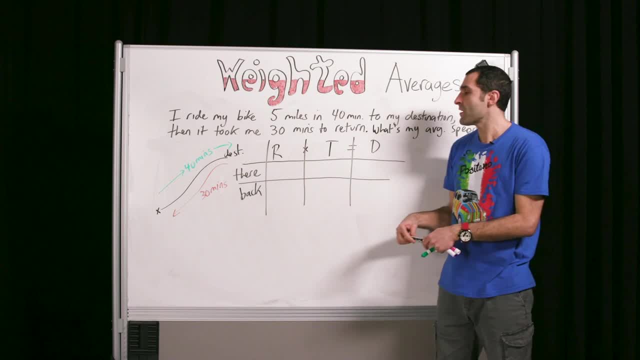 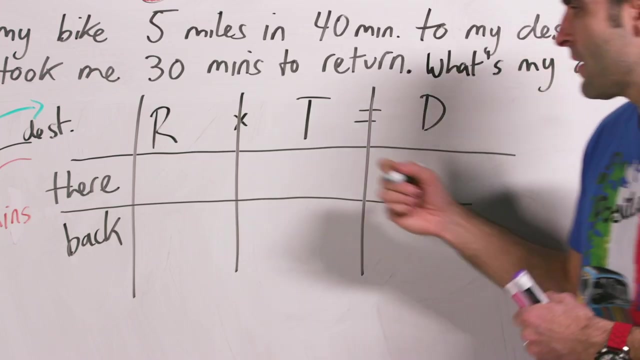 because then we can make our speed like miles per hour. So what we need to do is we need to convert minutes into hours, 40 minutes into hours. So 40 minutes is more than half an hour. What you could do- I'll pick green this time- is you could say it's like 40 over 60.. 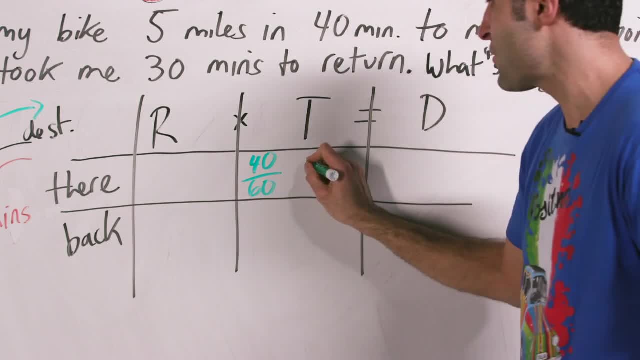 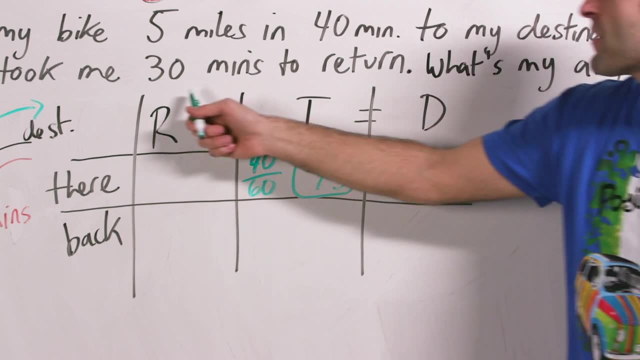 That's the fraction of an hour. 40 minutes out of 60 minutes is two thirds, two thirds of an hour. there It's 40 minutes, 30 minutes. on the way back It's a little more straightforward: 30 minutes, maybe you know. 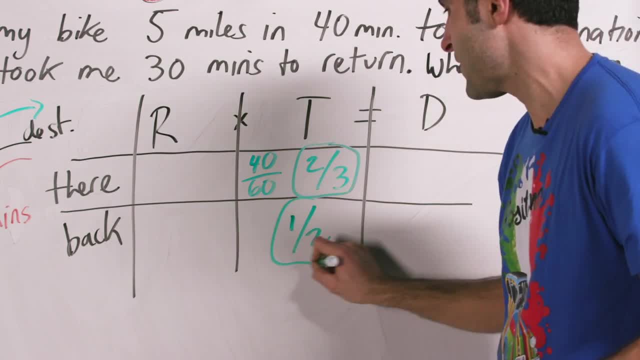 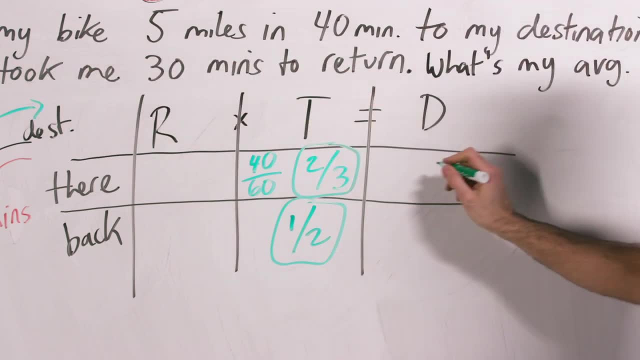 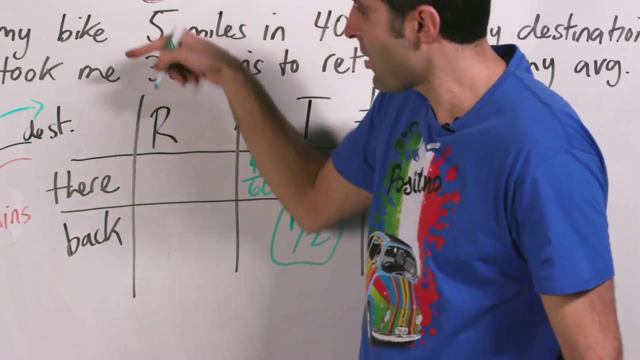 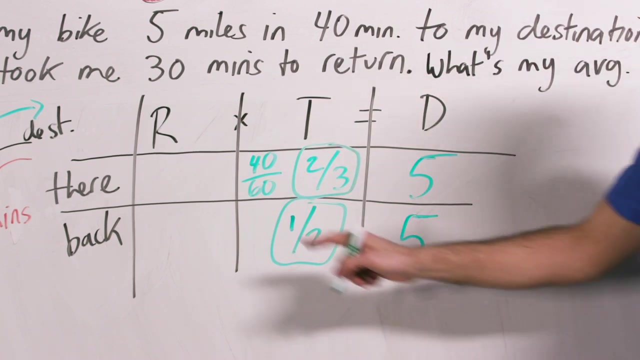 is half an hour, So I could put one half here. Let's box it so we could see it. Okay, What else do we know? Boom, I know distance: Five miles there. Did our destination magically become farther away when it's time to go back home? No, Five, All right, I don't know my rate there. 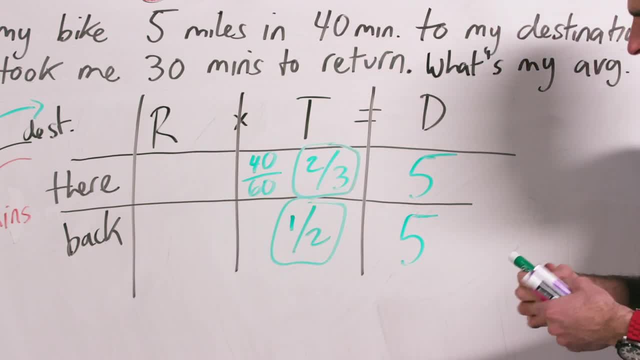 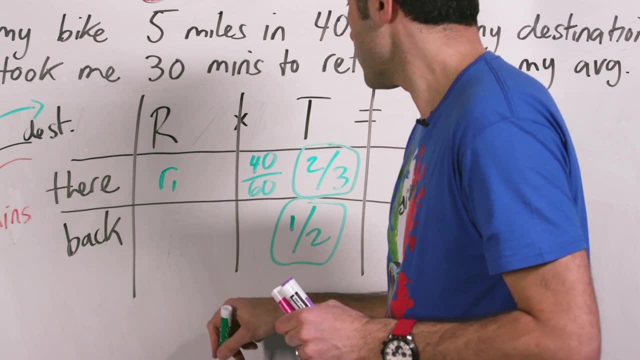 I don't know my rate back, But let's get it, Let's get it, Let's call it. you know, like um, you could say R1.. You could say R2.. You know you could do these things. 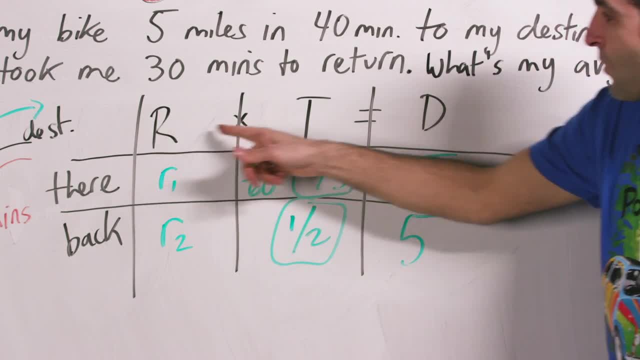 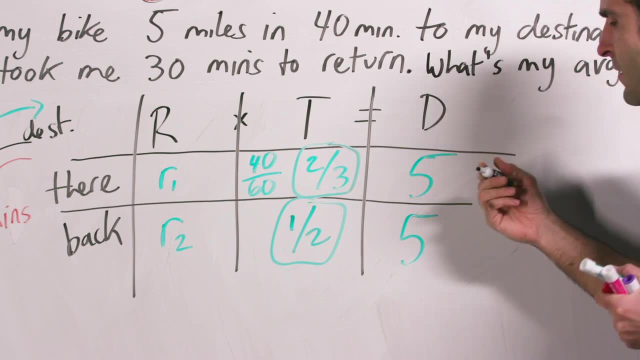 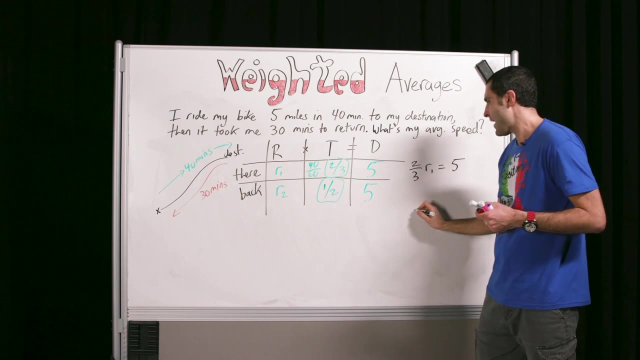 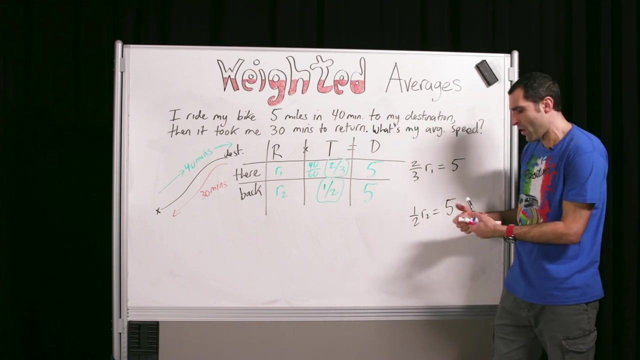 for our information. All right, Let's follow the formula, just like we did the last problem. Rate times time equals distance. So here we go. That would mean two thirds times R1 equals five, And then we have one half times R2 equals five. All right, Solving for R Multiply by reciprocal. 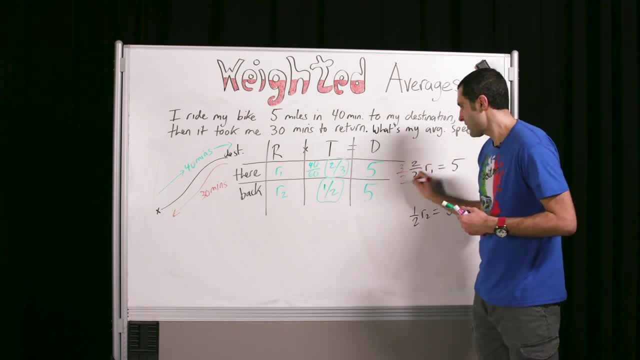 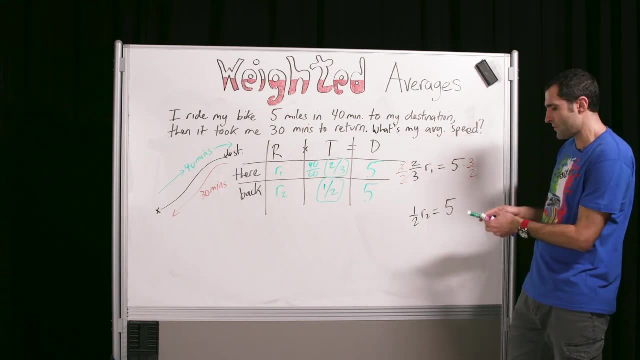 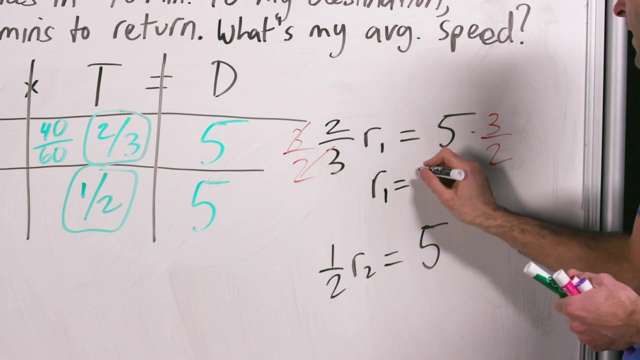 Let's go ahead and do that in red here. Times three over two, Times three over two, Down, down, down down. That's R equals 15 over two, 15 over two. So that's that first rate is 7.5.. 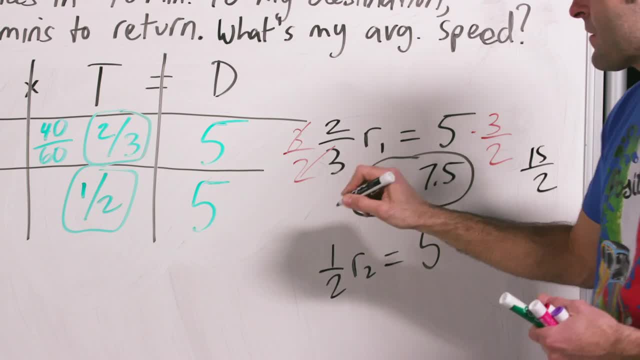 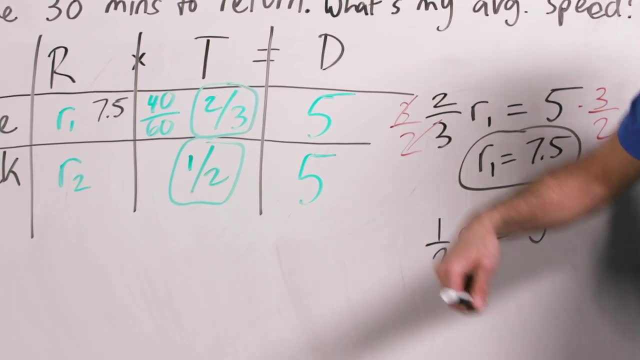 It's 15 over two. All right, Let's put that down: 7.5 miles per hour. on the way there It looks like on the way back we're going to go faster because we're going like downhill Takes us less time. 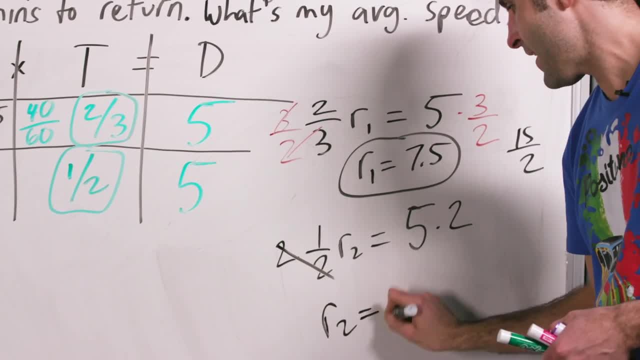 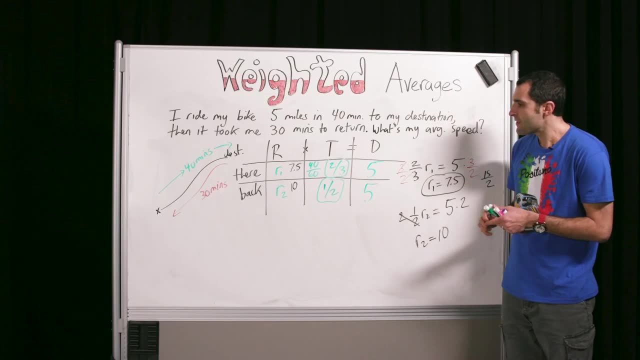 Lo and behold. if you hit that, R2 equals 10.. Yeah, We're going faster on the way back, So it's 10 miles per hour on the way back, Okay, So again, we can't just average these. 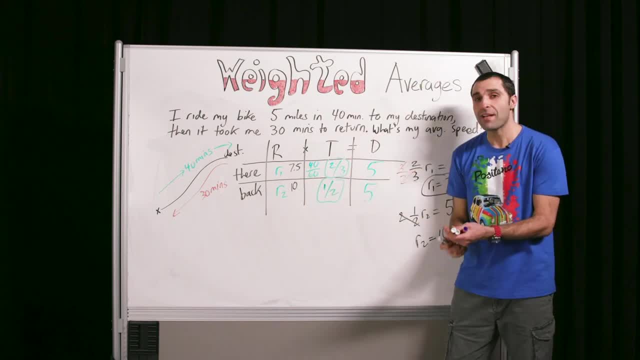 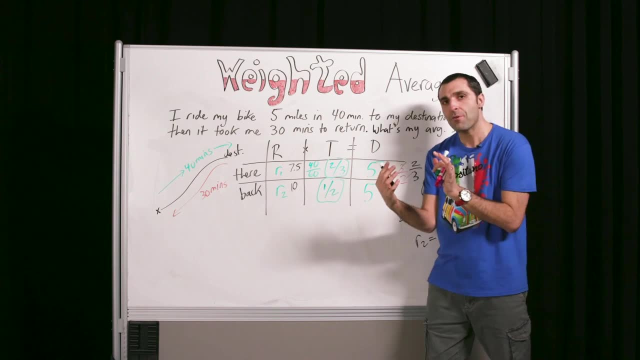 If I want my average speed, I can't average them. This is what I need to do. If we need to weight them differently, they need to have sort of like different power, And if they're going to have different power in our equation, we have to just add them up as they are. 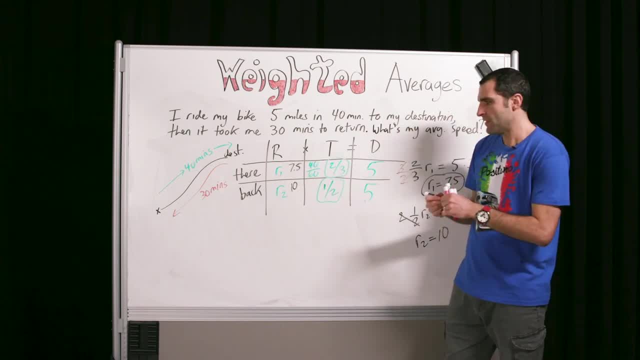 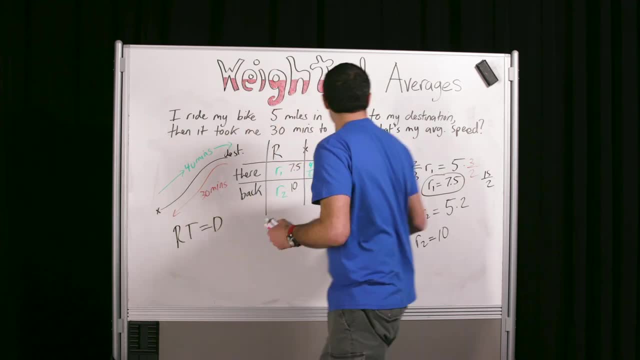 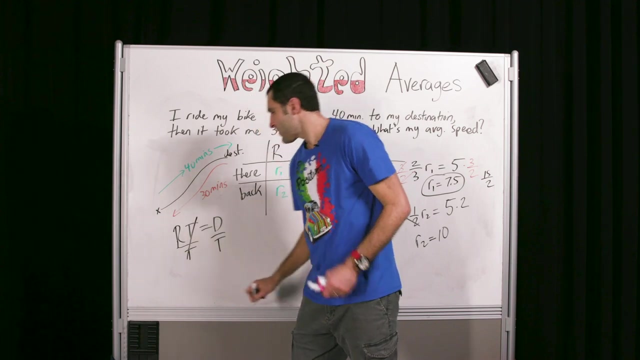 Here's what I mean. If R times T equals D, observe Here's what I mean: R T equals D. Now, since I want a speed, let's get R by itself by dividing by time. So essentially the rate will be the total. 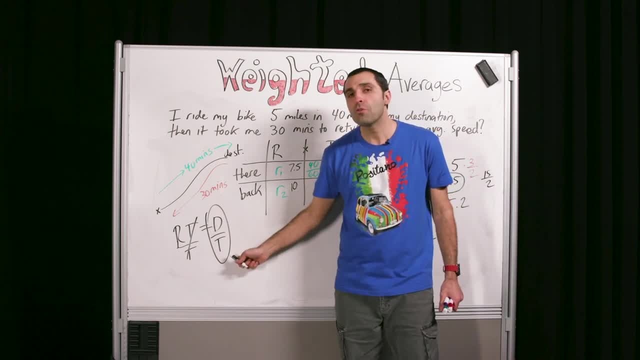 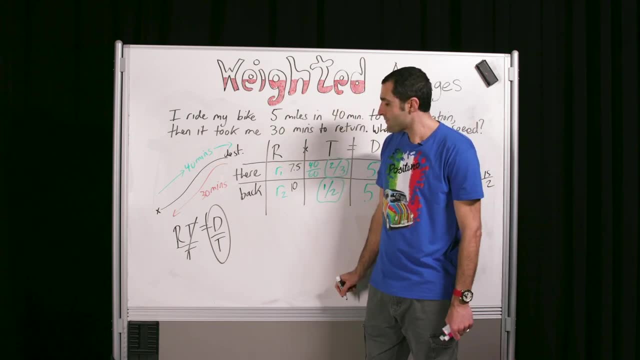 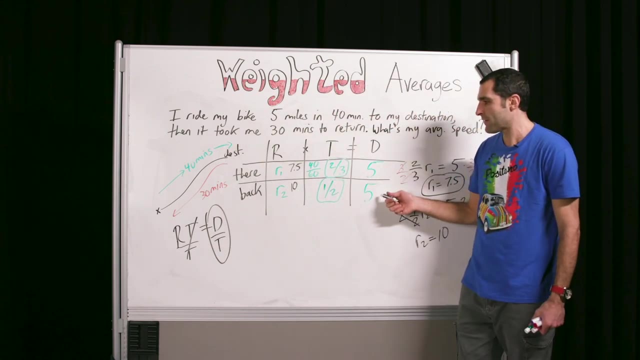 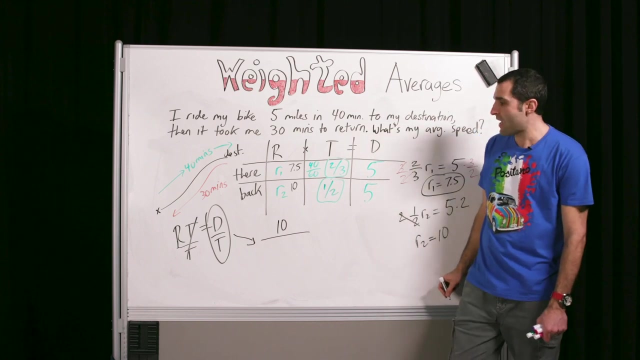 Total distance and the total time it took to get there. The total distance and the total time it took to get there, Okay. So let's try it. The total distance overall, okay, was five there, five back, That is 10 over. The total time collectively is two-thirds of an hour plus. 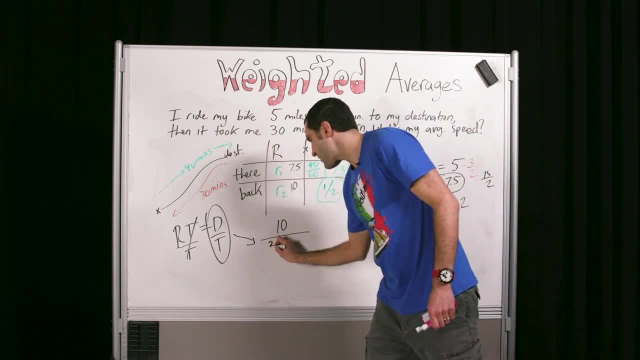 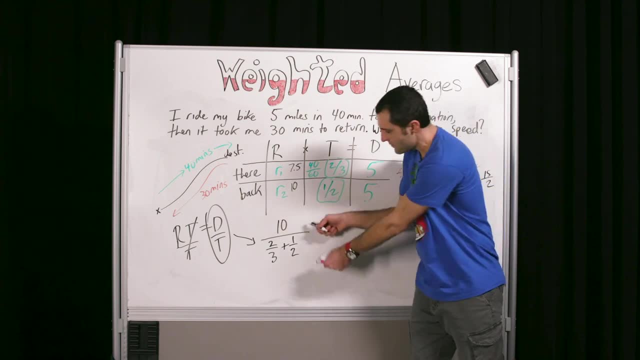 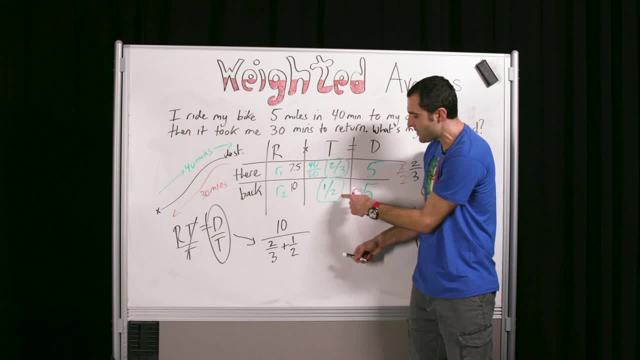 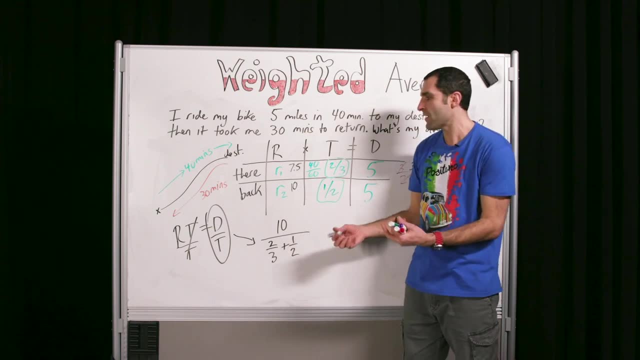 So now each of these are weighted differently, Like the two-thirds and the one-half are now equally- well, not equally, but like they each have some sort of influence in the equation, instead of simply averaging something that took different time to do. 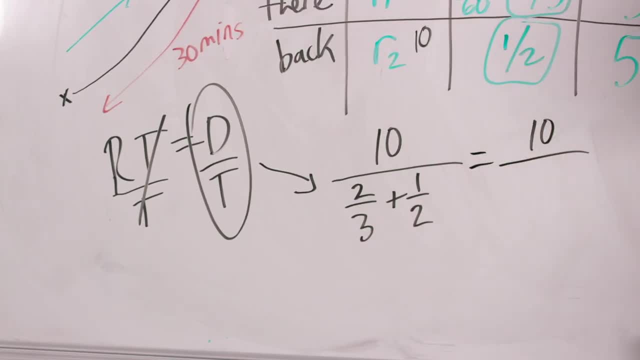 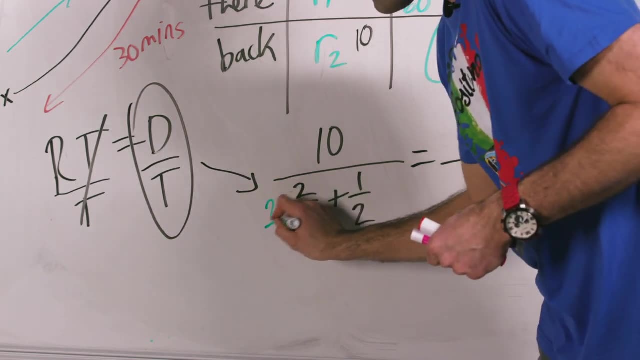 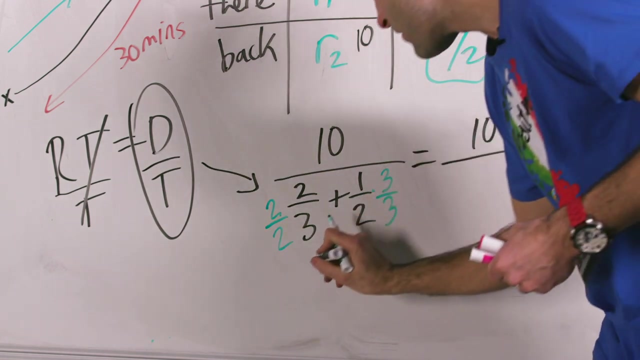 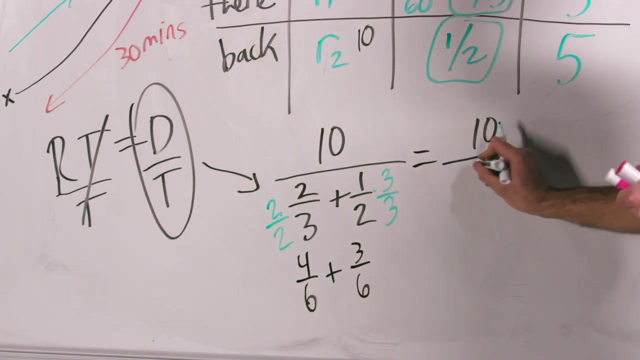 So here we go: Ten over Common denominator would be six in this case. So this would be times two, top and bottom. This would be times three, top and bottom. That's what we got, Four over six, plus three over six, And that's seven over six. 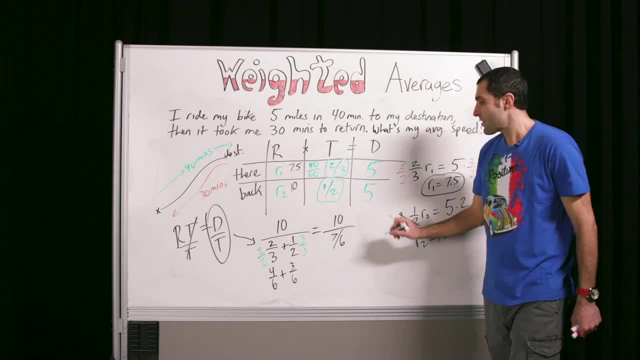 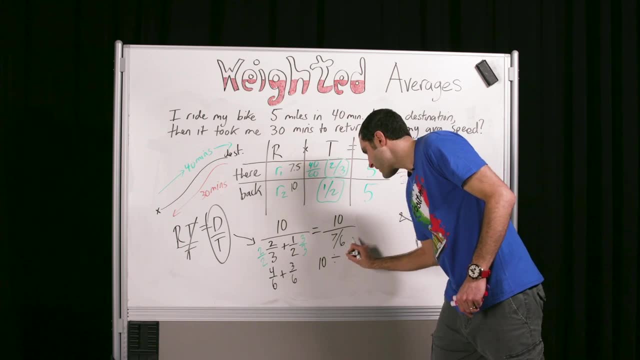 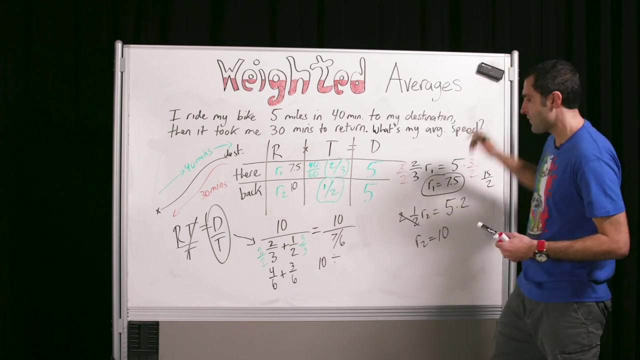 All right, Good job, And so what we can do in this case is: this is the same as ten divided by seven over six. Actually, I like the vertical fraction. You'll see what I mean: Ten divided by seven over six. 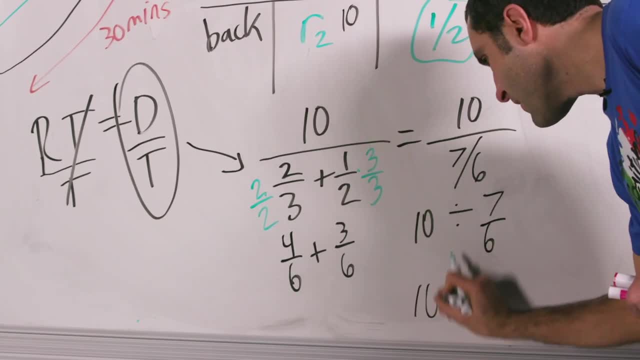 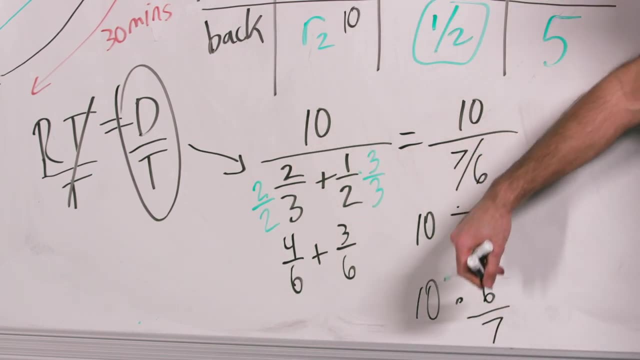 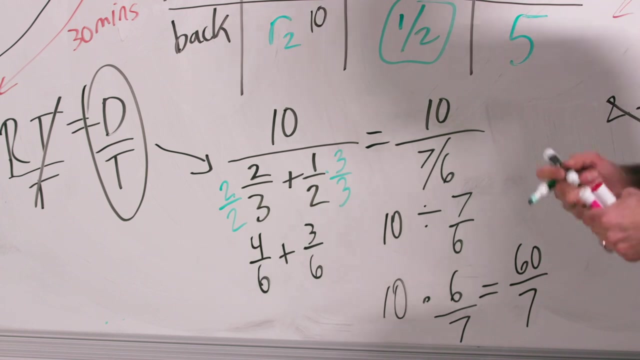 which is the same as ten times the reciprocal six over seven. So dividing by a fraction is the same as multiplying by its reciprocal. Multiply across, we get sixty over seven. Now that's not really meaningful until we get it in speed which is measured in miles per hour. 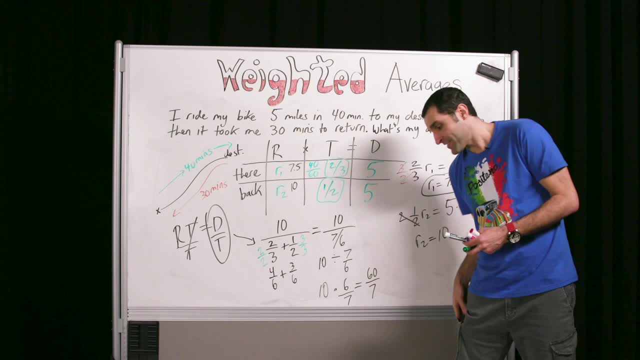 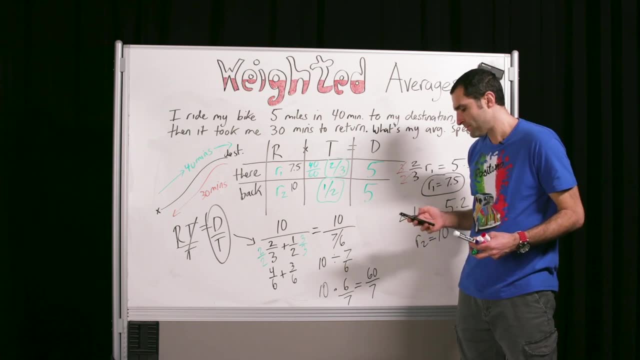 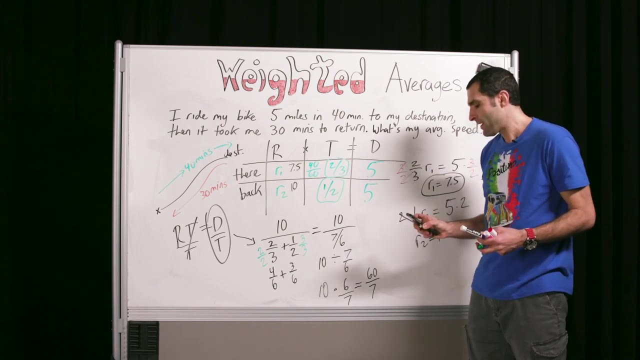 So let's get the handy-dandy personal calculator. Unlock it, Unlock it, Boom. We got sixty over seven. Eight point six Rounded, Eight point five, seven, I got, But eight point six, Eight point six. And now let's confirm. 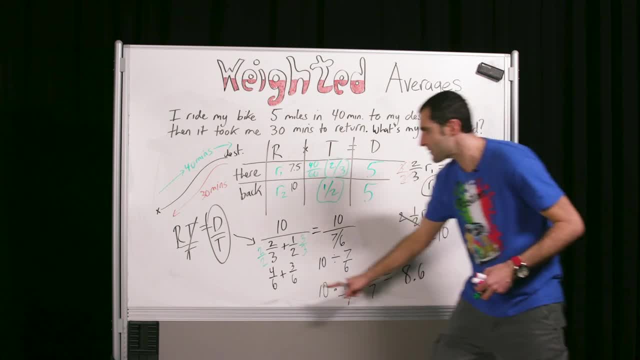 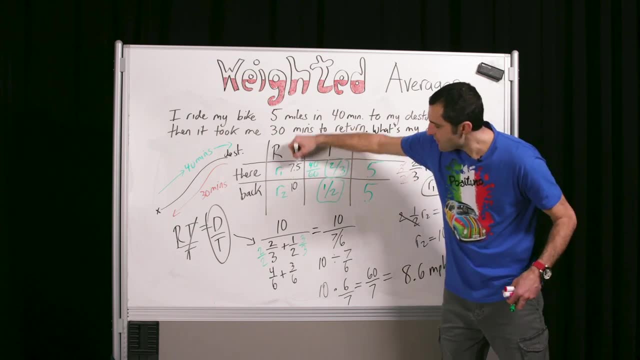 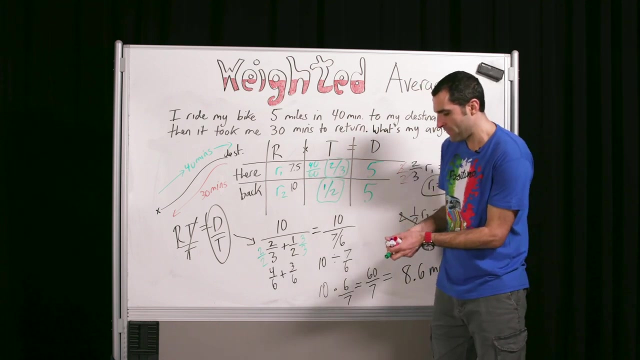 If this is a rate, an average speed, that's miles per hour, And we have to look and see Eight point six is indeed closer to the seven point five. So that's one of the reasons we got eight. point six is between these two. 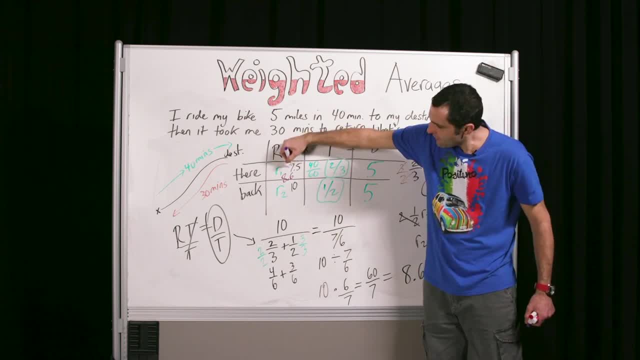 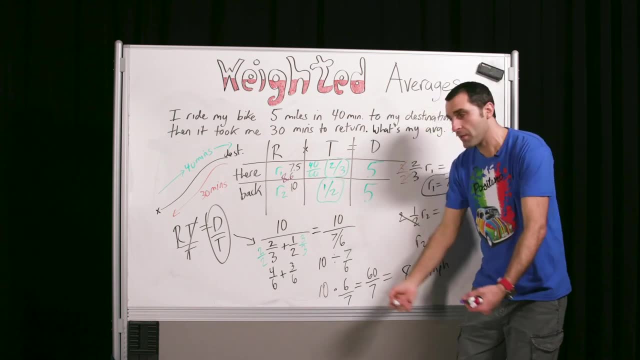 My speed. there is seven point five. That's like one point one away, One point one away, And this is the same thing. This is one point four away. So you could see my speed was like slower because I was doing this for a longer amount of time. 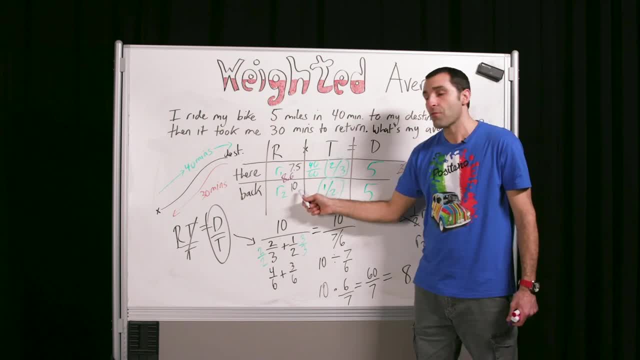 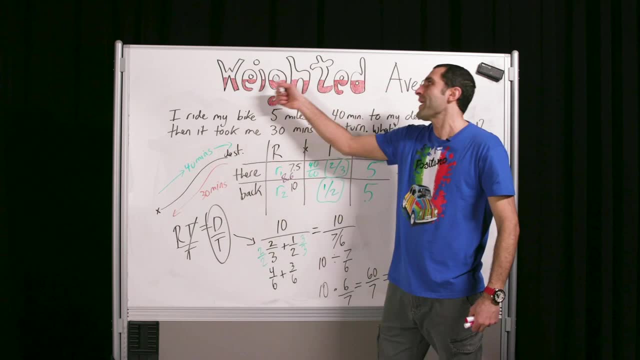 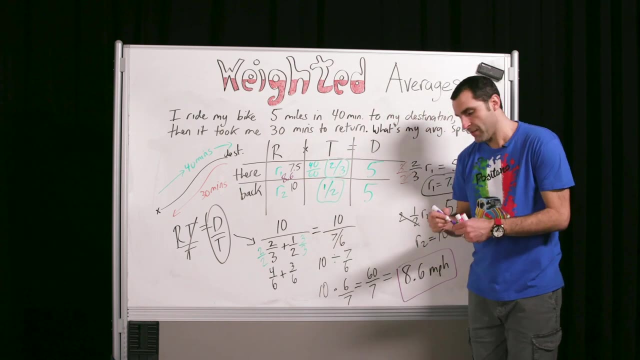 I was doing this for forty minutes, where I was doing this for only thirty minutes. So that slow time it took to get there had more of an influence, had more of a weight on my average speed. So that's why it's eight point six miles per hour. 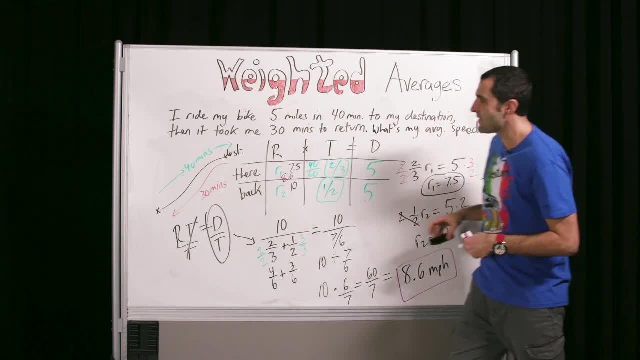 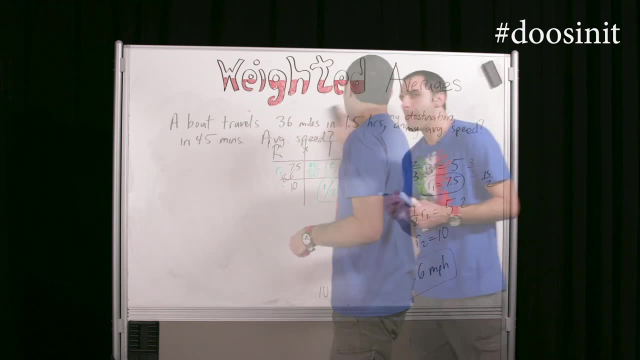 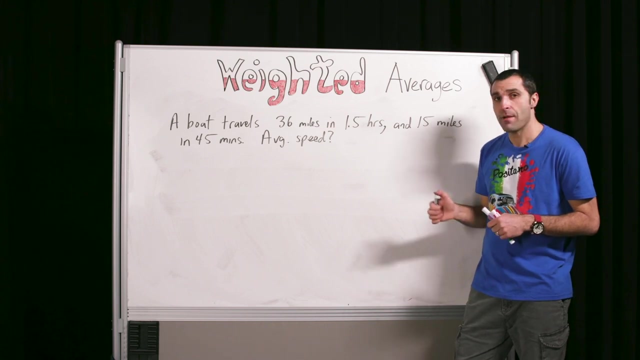 Nice work. That's a doozy. A doozy And we dooznit. I don't know what that means. Okay, Last one of this particular lesson. Okay, A boat travels thirty-six miles in one and a half hours and fifteen miles in forty-five minutes. 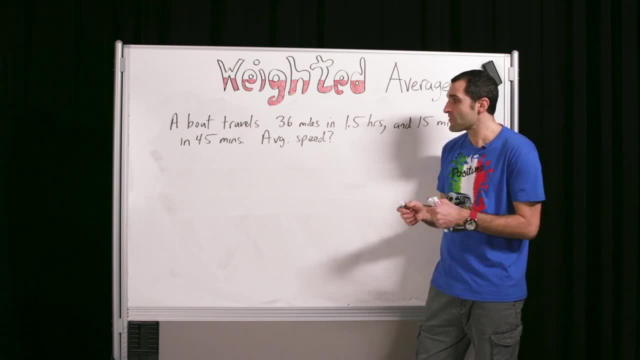 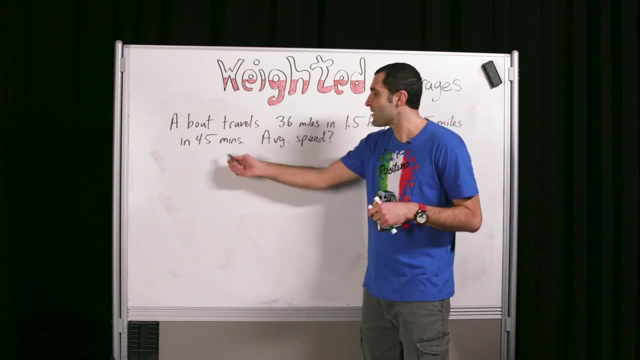 What was the average speed? Okay, So this is similar to the last problem. We have a little bit of curveball here. We see, one time is given in hours And the other time is given in minutes, So we should sort of make them both into hours. 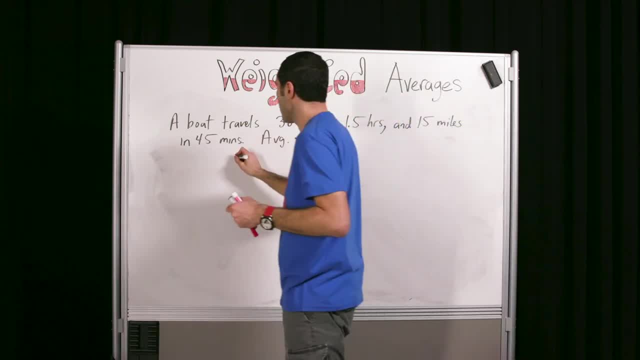 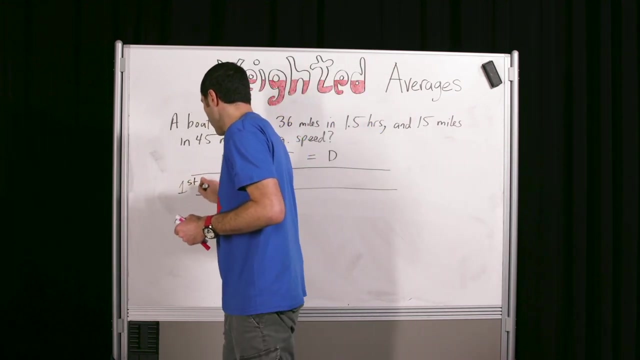 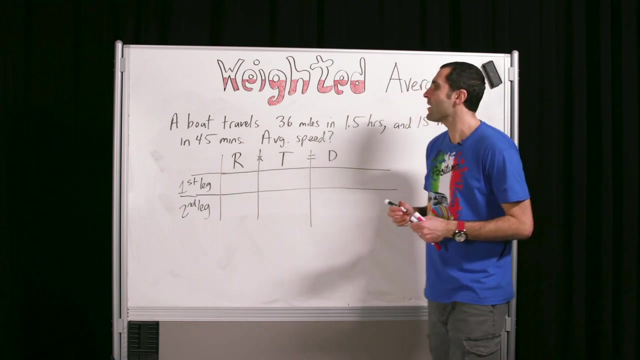 And we can get that average speed. So here we go. So rate times, time equals distance. Here we go, All right, So we could say first leg, second leg of the journey, Okay, What do we know? What do we know? 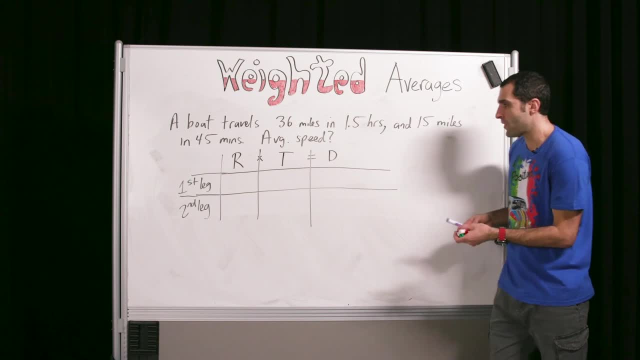 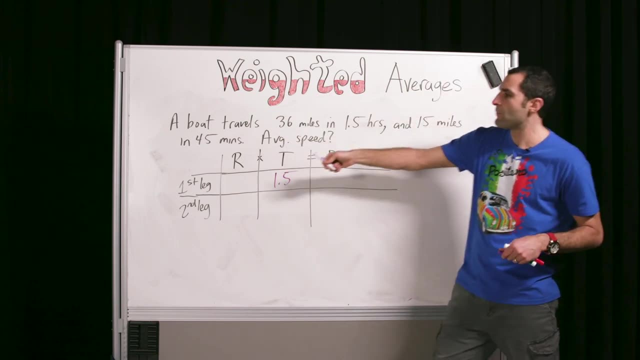 We know the time in the first leg is one point five. It's kind of fun. You just fill in what you know And then it'll open up. We know the time. Oh, over here, Forty-five minutes. We're going to turn that into hours, just like we did last time. 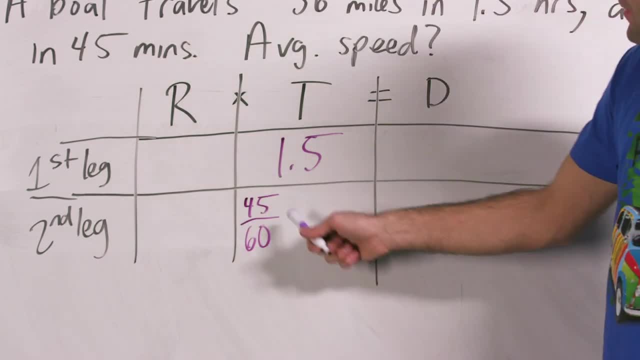 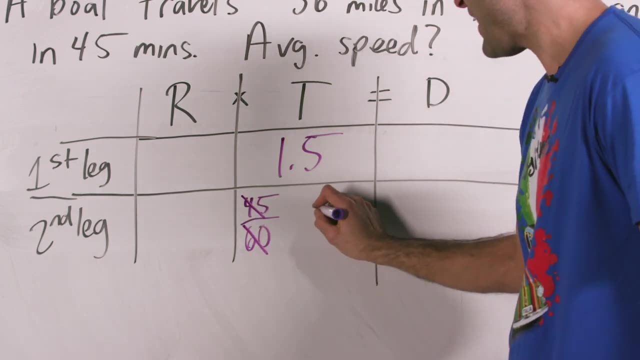 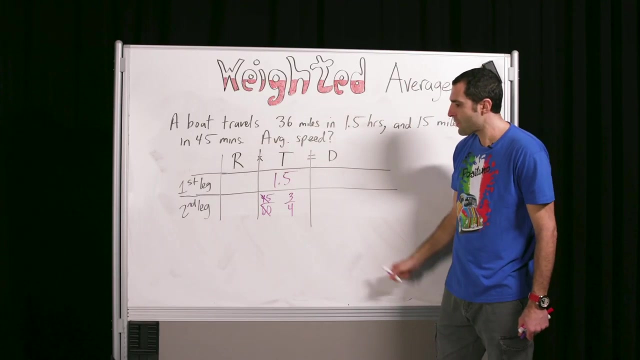 Forty-five over sixty minutes. Maybe you know that forty-five is three-fourths of an hour. Forty-five minutes Or divide top and bottom by fifteen And you get three over four. In fact, if we want to go to consistency for decimals, three over four is point seven-five. 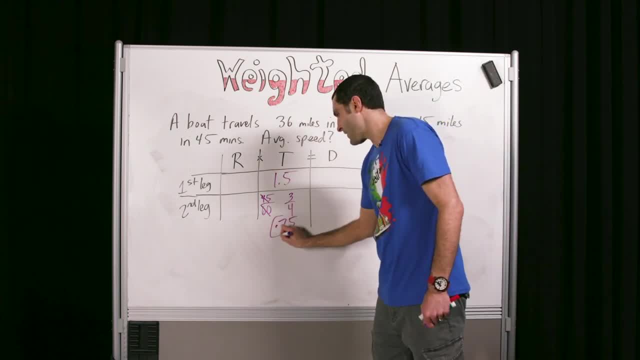 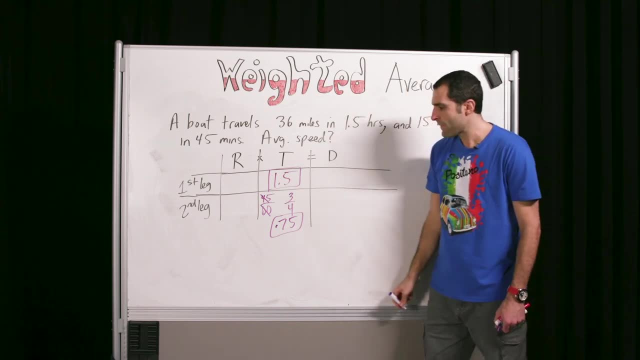 So let's just do that one Point seven-five, Just leave it at that one. Okay, Good Notice, we're just figuring it out as we go, okay. So we don't know how fast it was going the first way. We do know the distance. 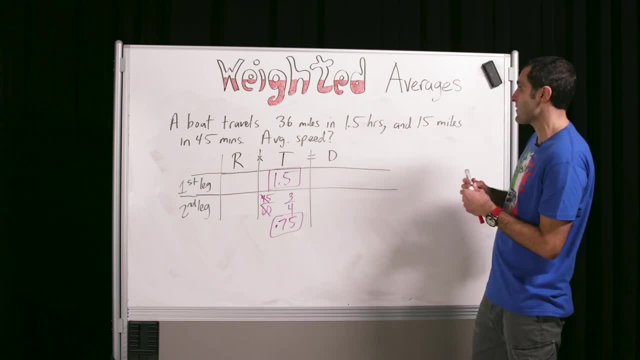 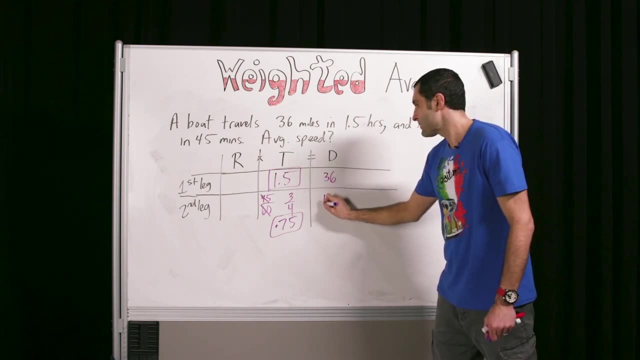 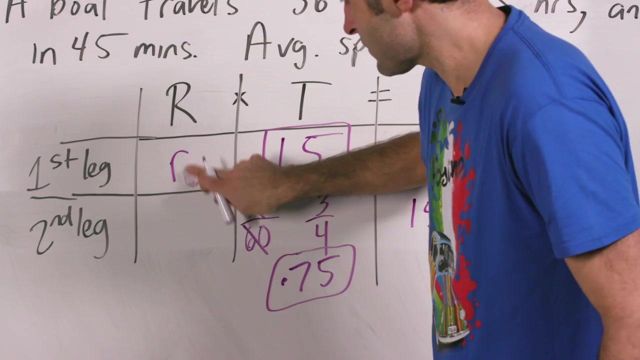 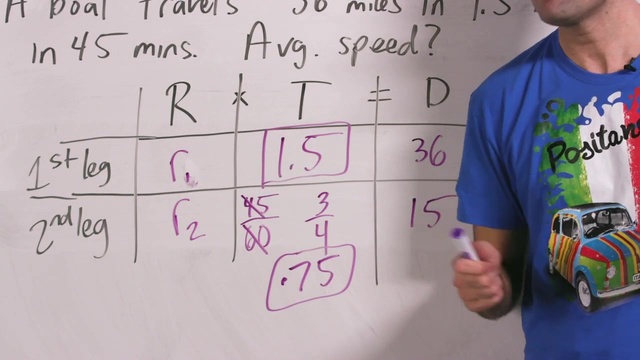 Do we know the distance? Yes, We know thirty-six miles And we know fifteen miles. Okay, And again, this was R1 and R2.. Last time, last time, we solved for these rates. Maybe you noticed that we didn't need to. 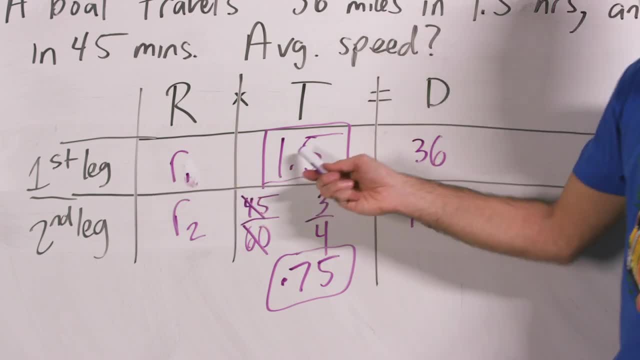 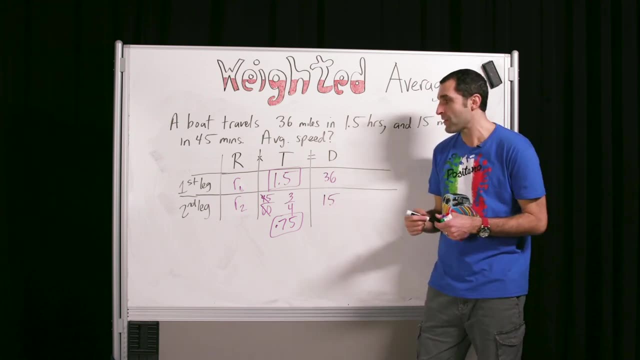 It's nice to, and you saw how, by multiplying R times 1.5 equals 36, and so forth, solving for R. But what we can do instead is just. What we can do instead is just go straight for the average speed, now that we have our. 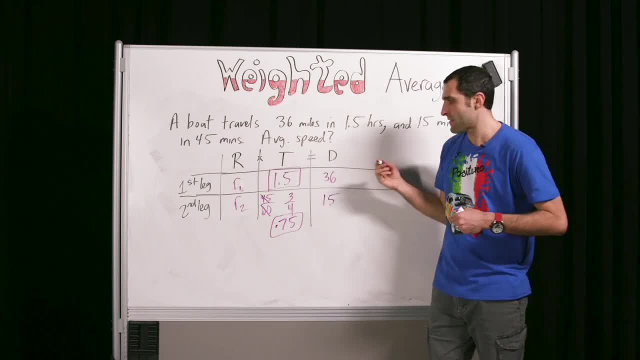 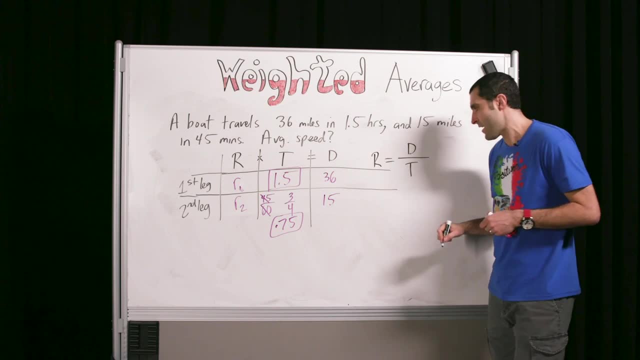 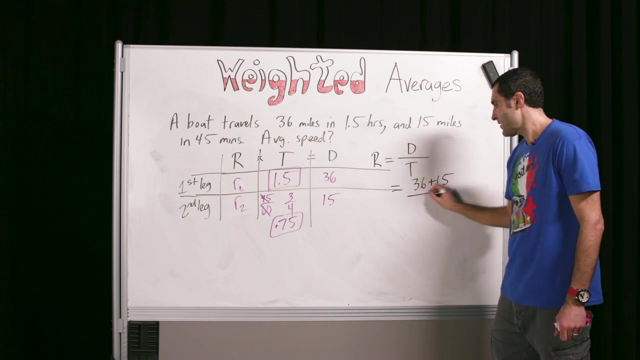 sea legs, you know. So let's do this. So the rate is the overall distance over the overall time. Total distance: thirty-six plus fifteen. Total time: one point five plus one point seven-five. That's it. That's it. 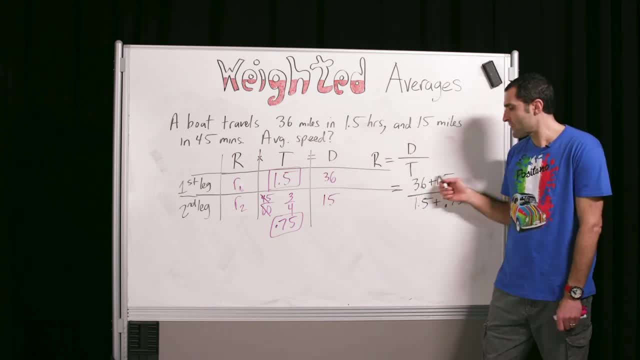 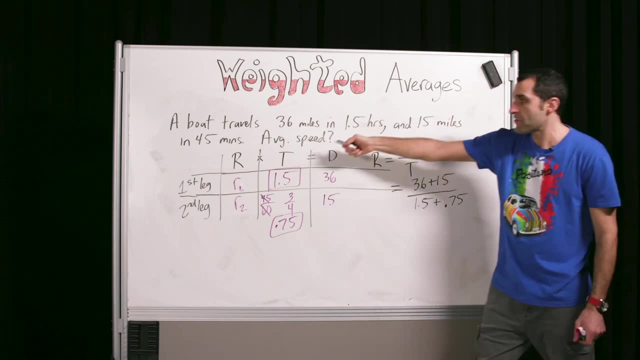 That's it. That's all it is. Look at that, It's so cool. Your total distance and the total time it took, that'll give you your overall rate, Your average rate, Your average speed, That's what it'll give you. 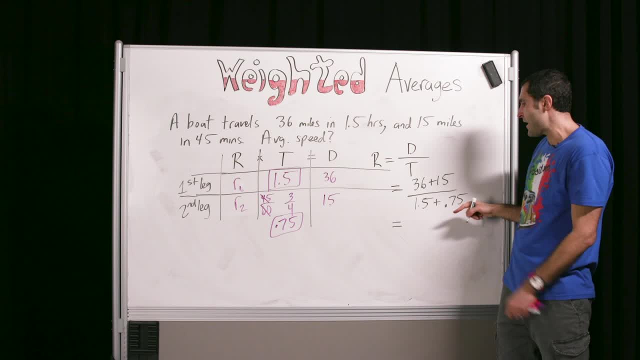 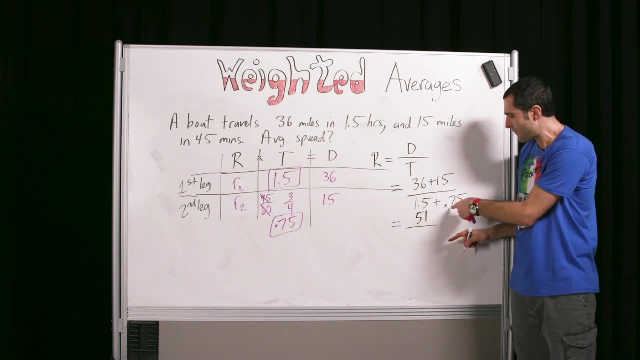 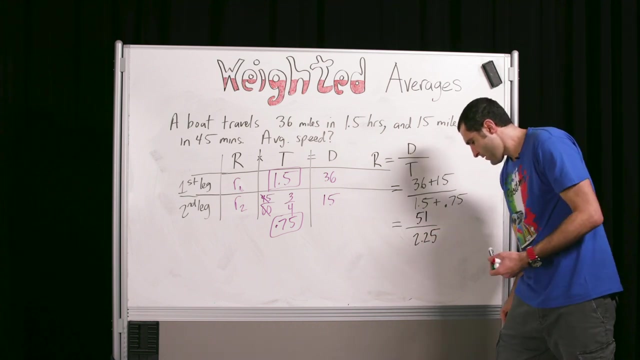 All right, Rockin' and rollin'. These two together make forty plus eleven fifty-one. These two together make one and a half plus point seven-five. this is two point two, five. All right, Set it up. Set it up. 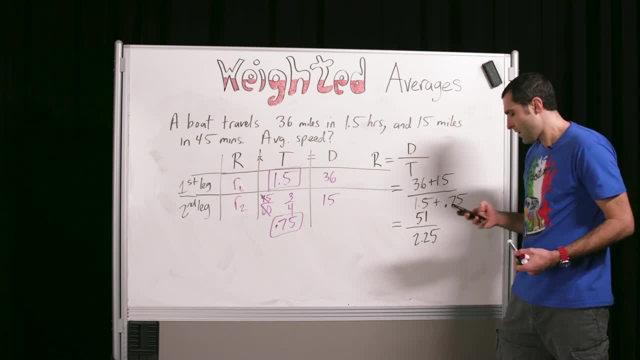 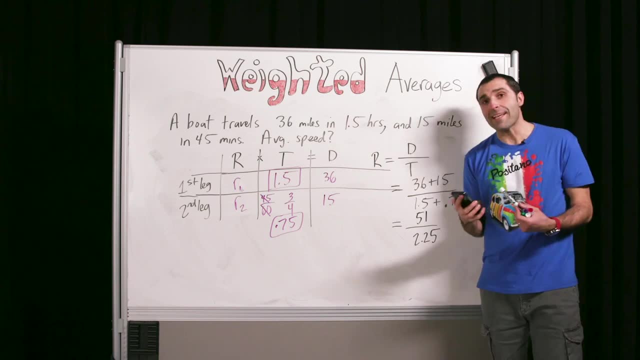 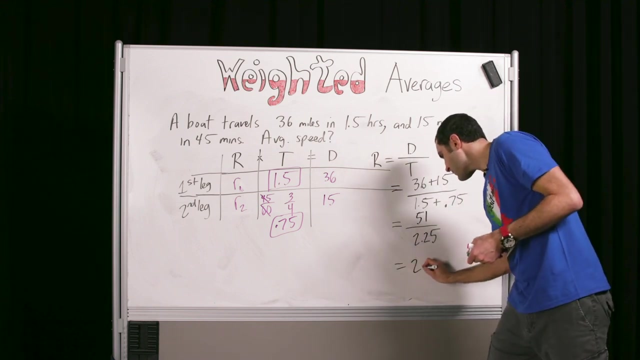 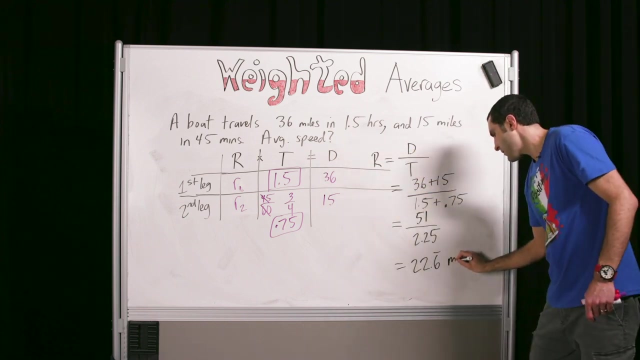 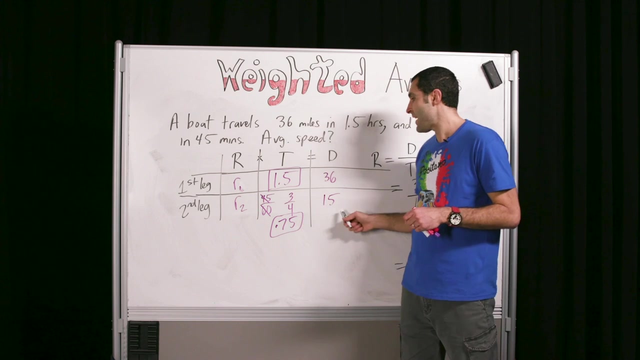 Set it up today. Set it up today: Fifty-one divided by two point two, five. Twenty-two point six, repeating, Twenty-two point six repeating, And that is a rate And that is in miles per hour. Okay, So it turns out that if I travel thirty-six miles in one and a half hours, then it takes 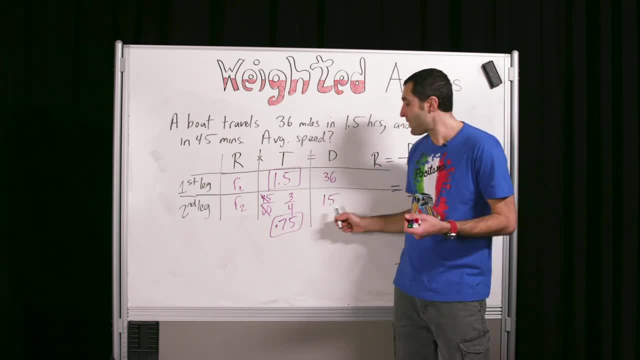 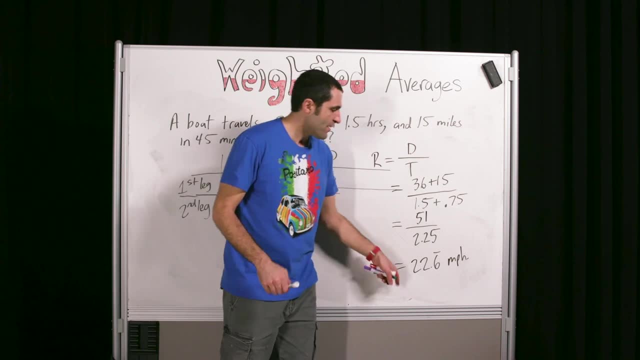 me three-quarters of an hour to go, fifteen miles overall. the average is twenty-two point six miles per hour was my speed. All right, Good job. I hope you like this. You know, I sort of got into the flow of it. 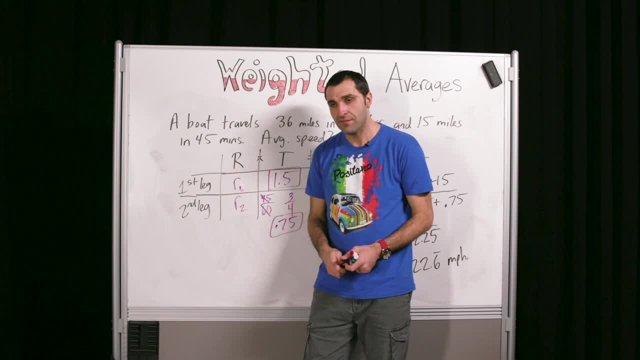 I wanted to do that, so you got into that flow as well. So, thank you, Thank you, Thank you for committing to this process with me, Yay math.